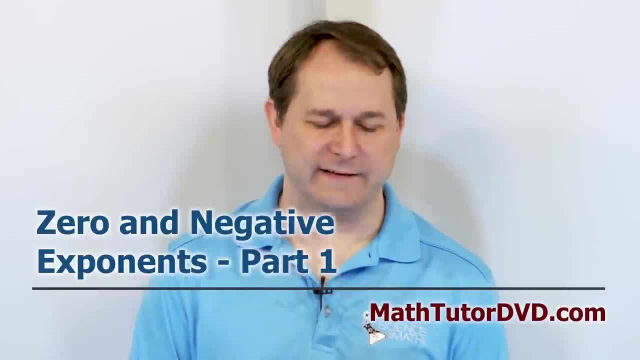 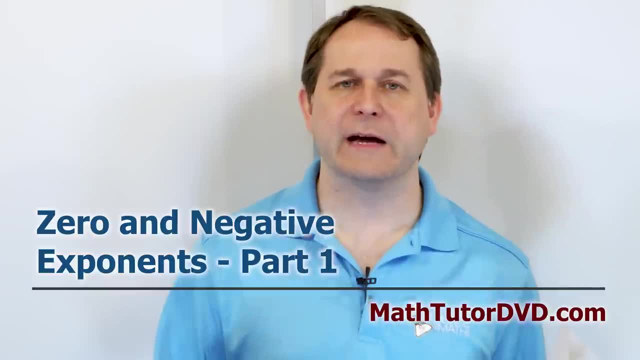 Hello, welcome back to Algebra. The title of this lesson is Zero and Negative Exponents, Part 1.. Now I get excited about teaching certain lessons, and this is one of them. actually, because I remember when I first learned the concept of an exponent, Something raised to. 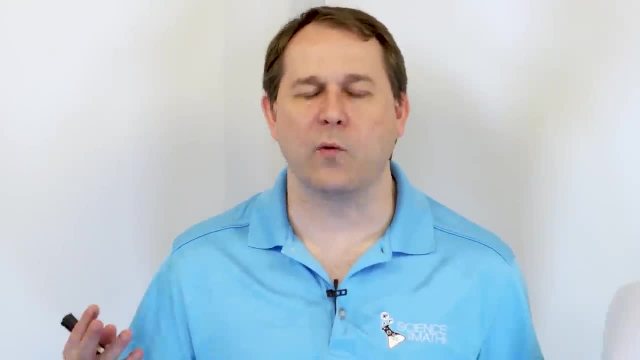 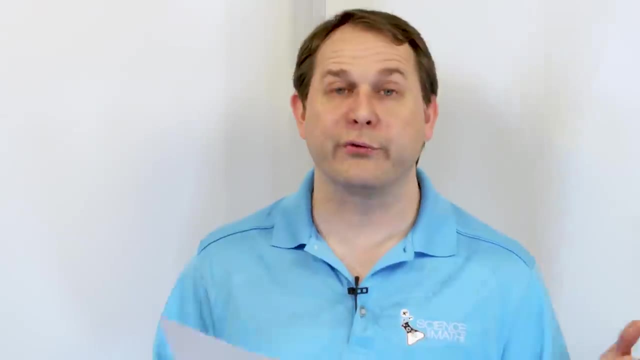 the zero power didn't make sense. Something raised to the negative one exponent to me at the time didn't make a lot of sense because I can visualize three to the power of two. Three times three is nine, but I can't visualize three to the zero power. That doesn't make sense and I also can't. 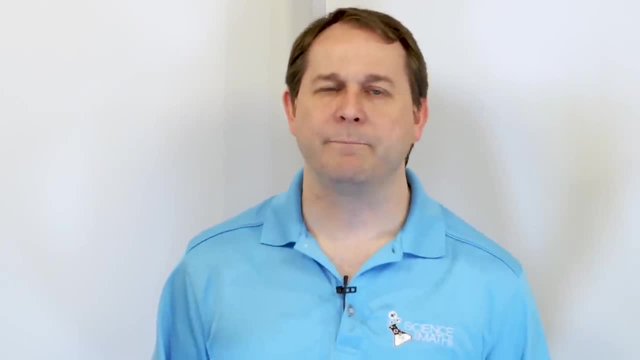 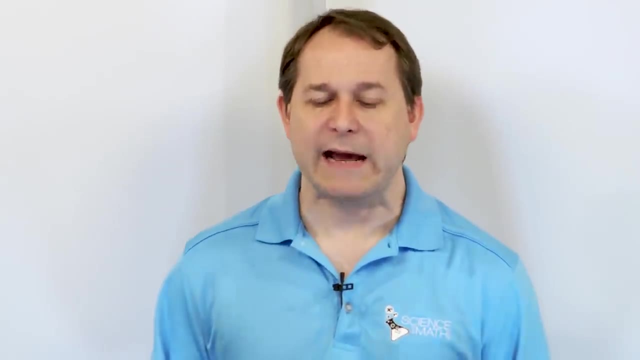 visualize very easily three to the negative five power. So what we're going to do in this lesson is we're going to talk about these rules that involve zero, exponents that are zero and exponents that are negative, And I'm going to write those rules down and we're going to talk. 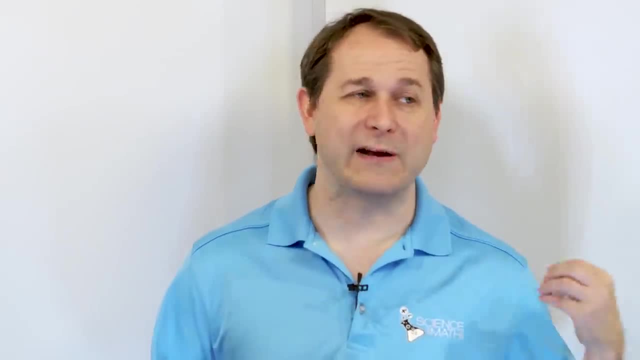 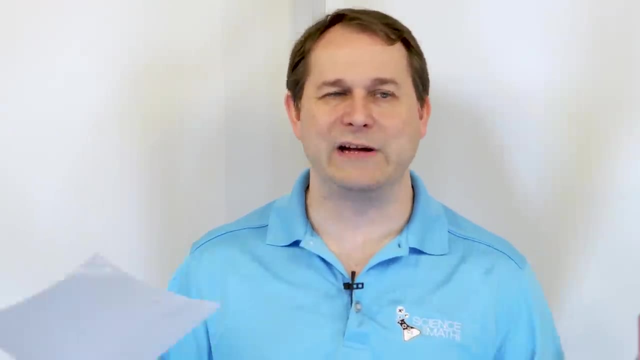 about them, and I'm going to actually show you where those rules come from, because when I first learned algebra, nobody told me where they come from. I just had to learn them, right, And it's just one of those rules you have to learn, you have to memorize, but you don't have any idea. 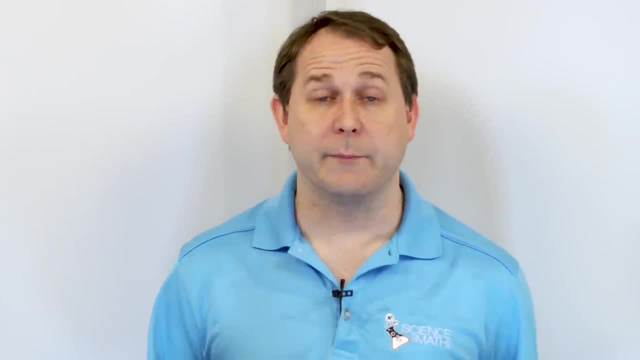 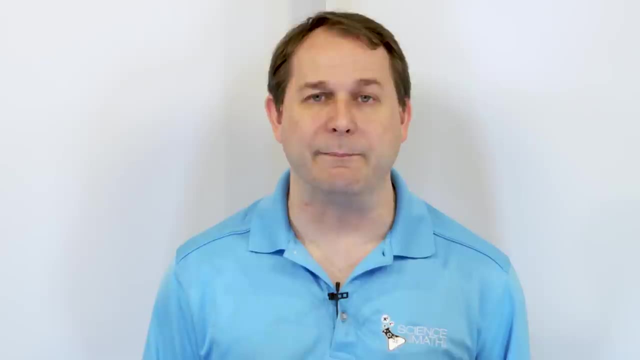 what it means. We're going to talk about what it means and where it comes from here, and then at the end we're going to do several problems to give you practice with zero and negative exponents, and then we'll have more complicated problems in the next lesson. So before we get too far into this, let's write. 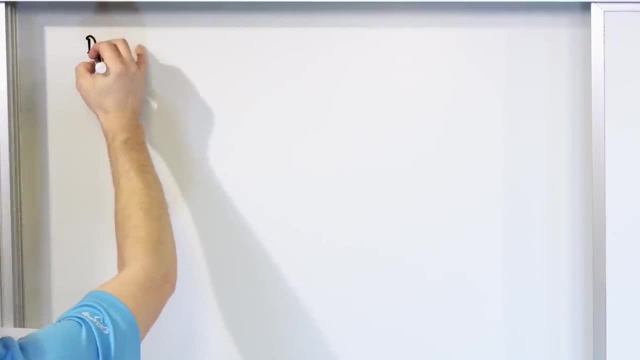 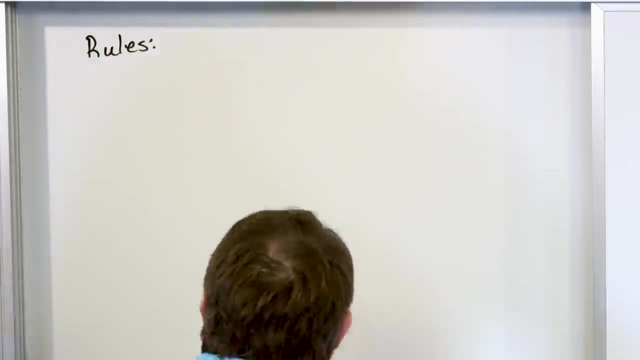 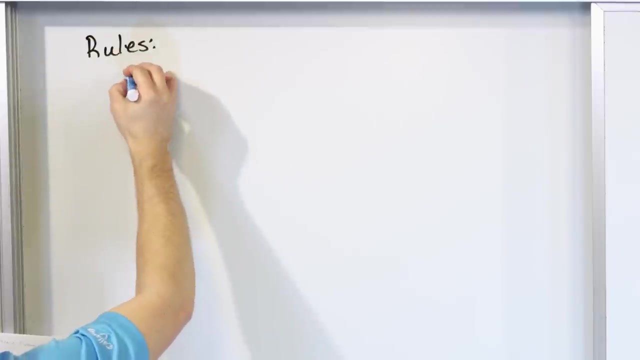 down the two rules that we have for zero, or at least the two basic rules for zero: exponents that are zero and exponents that are negative one, And those go as follows: Any value of a variable number, whatever a raised to the power of zero is always, always, always, always, equal to 1.. So if you see an equation, 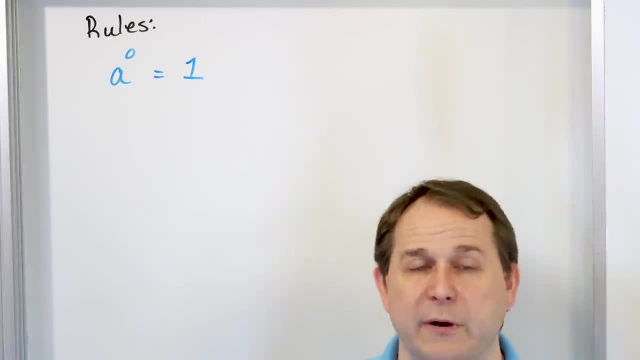 later on down the road, in calculus, trigonometry, algebra, anything. if there's a term raised to the zero power, you just say it's 1. You don't have to think about it, you don't have to manipulate it. 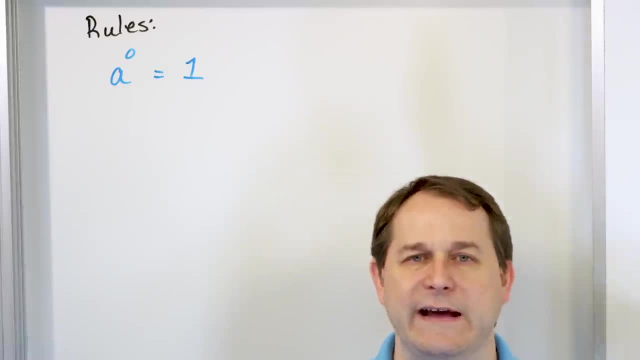 or show it. It's just a fact. It's something that we take to be true in math, that you don't have to prove every single time you use it, And I'm going to show you why in a minute. but this is a rule. 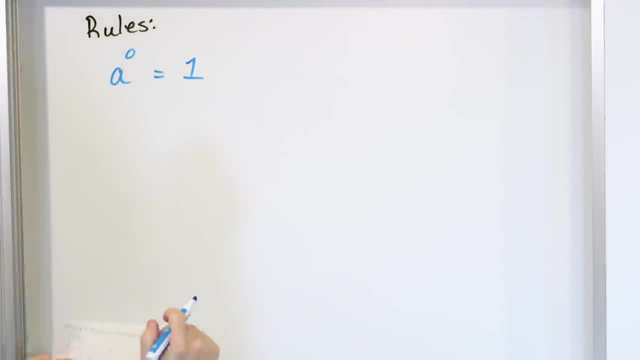 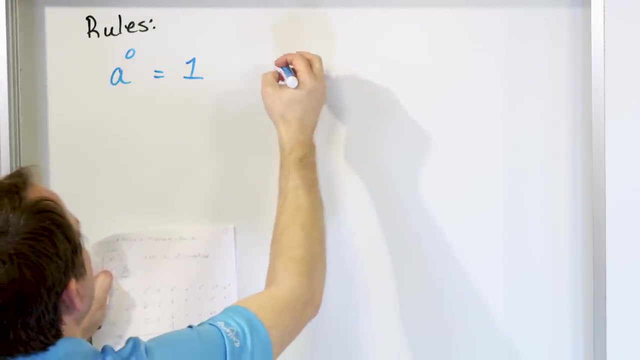 that you're just going to end up having to use all the time. And then we also have another rule. Oh, let me show you, tell you one important thing: When we say that a to the zero power is one, we are implying that the variable a cannot be equal. 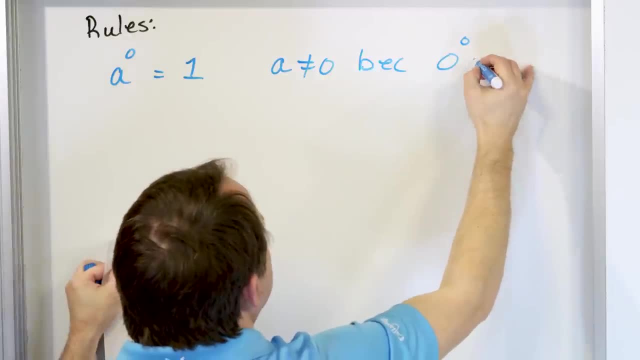 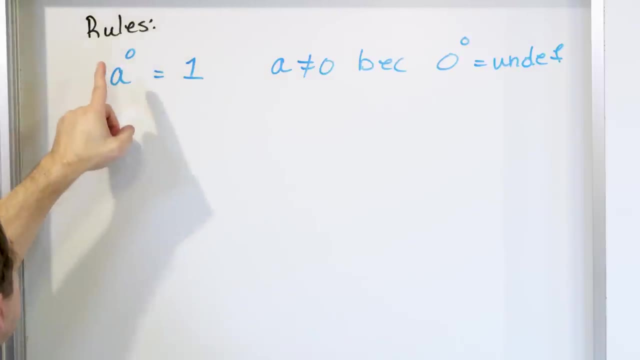 to zero, because zero to the zero power is undefined, So I should have said that before. So when I say a to the zero is one, what we're really saying is: you know, one to the zero is one, 16 to the zero is one, 32 to the zero is one negative. five to the zero is one negative, 64 to. 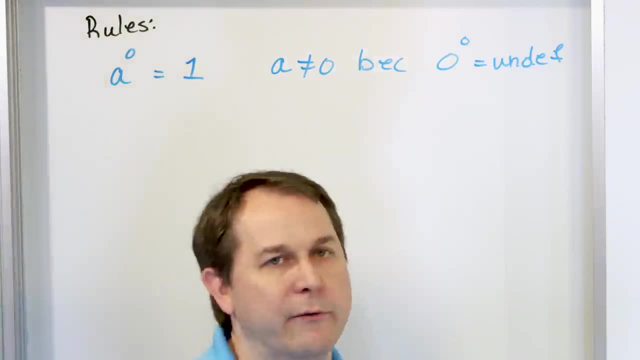 the zero is one. All that's true, but zero raised to the power of zero is not defined, And you'll see a little bit more why as we go through the derivation, why it's not defined. but you can't have an equation with zero raised to the zero power. Now the other rule that we have, involving 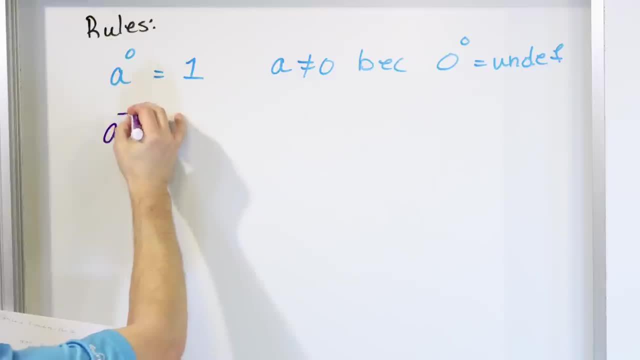 exponents like this is a base raised to a negative exponent- can always be written as follows: Just take that exponent- the base and the exponent- and move it to the denominator of a fraction and make the exponent positive. What this is saying is that if I have a negative exponent up here, 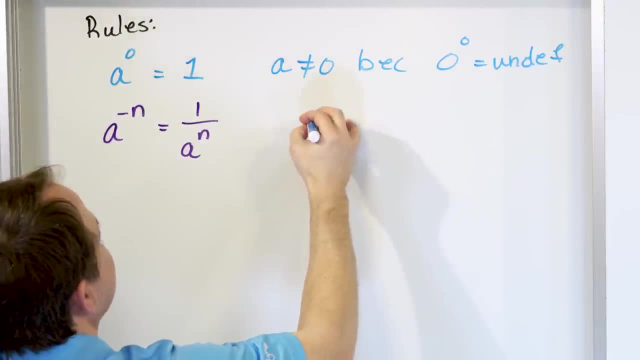 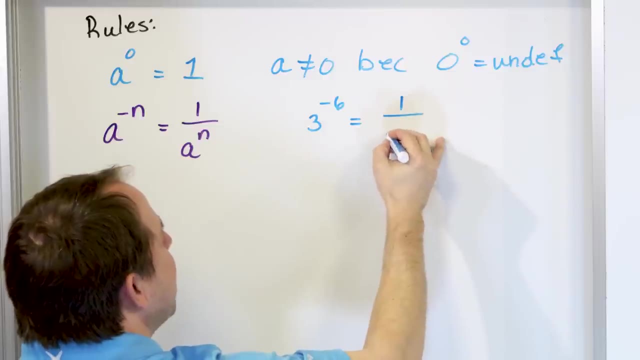 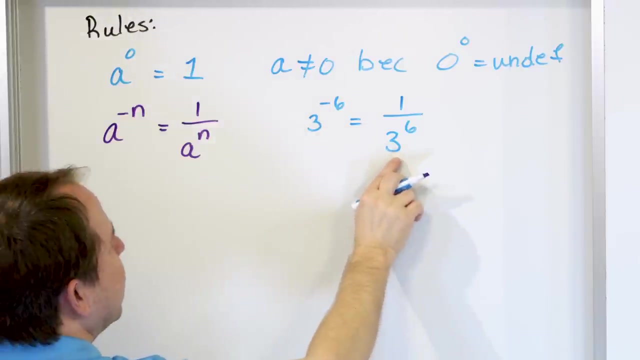 just to take a concrete example. for instance, if I have three to the negative six power, what it means is it's exactly the same thing as putting it in the denominator of a fraction with a positive version of the same exponent. These are, by definition, equivalent. So here I've written it. 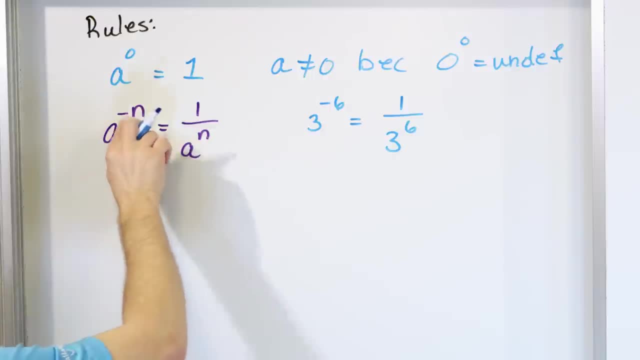 with the number three, but it applies to every exponent. So if I have a negative exponent, any variable, so x to the negative, n or y to the negative, n, whatever, or x to the negative six, x to the negative, five, whatever, you just put it on the bottom and make the exponent positive. 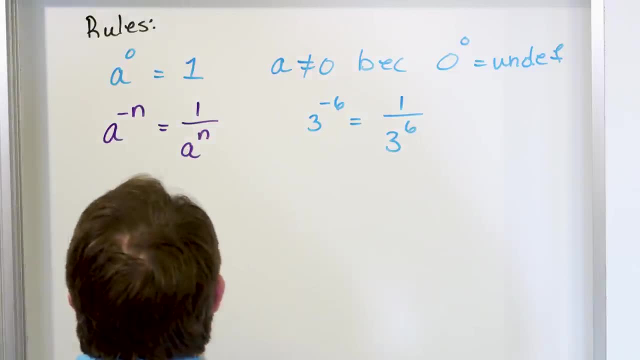 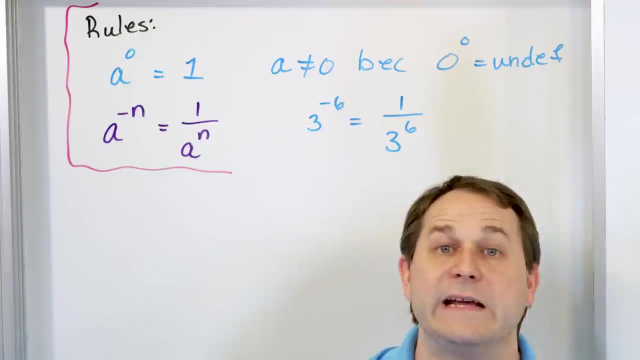 These are equivalent. So these are what we call the important rules of exponents. Well, there's lots of rules of exponents, but these are the rules that involve zero and negative exponents. And again, as I said, when I first learned these rules, someone said: hey, these are the rules. 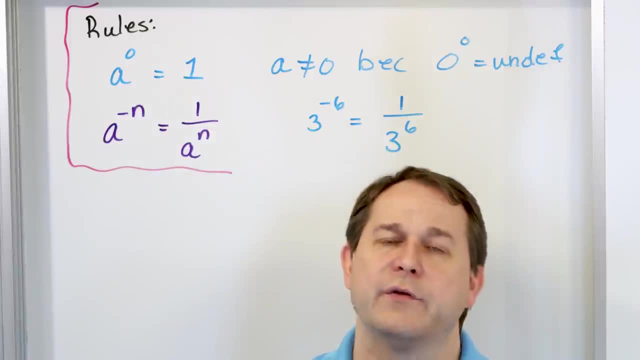 you have to use them, But I didn't understand where they come from, So I want to take a minute and then we will do some problems showing you how to simplify expressions that involve negative exponents, Because I know you may not believe me now, but you have to trust me. negative exponents. 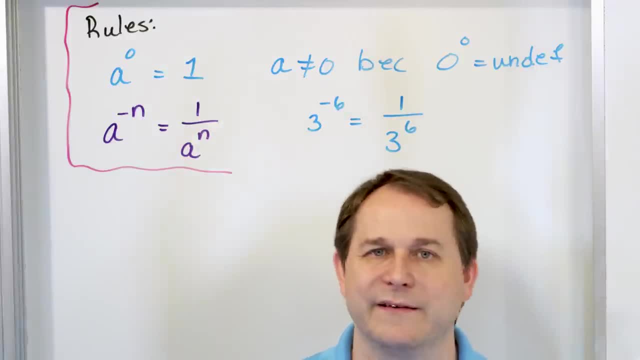 will be in your life forever. They're used all throughout: calculus, physics, chemistry, everywhere. Equations with zero exponents, equations with negative exponents are everywhere, So you're just going to have to get used to it. So let me start out. let me start out by a concrete example. 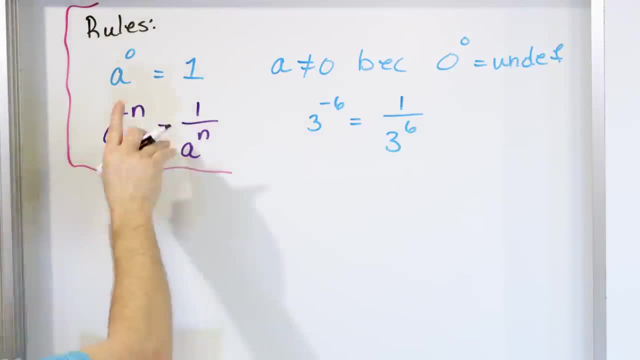 Let's take any number, it doesn't matter, because here I'm using a base of a. that's what you'll see in your book. Let's bring it to the next level. So let's start with a base of a, and I'm going to. 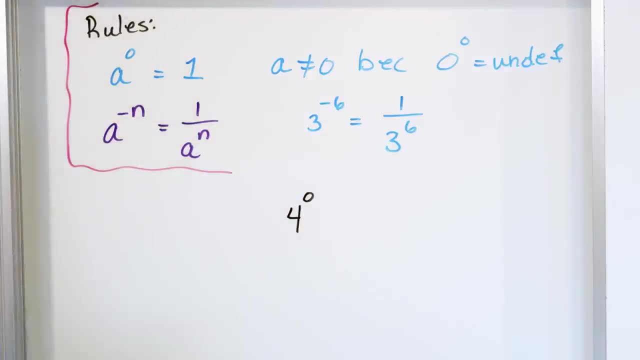 down to earth and say we have a number four to the zero power. Now I know that I just told you anything to the zero is one and it is. but let's just hold that in the back of our mind for a second. So we know we can have a zero exponent. We also know we can have the positive exponents. 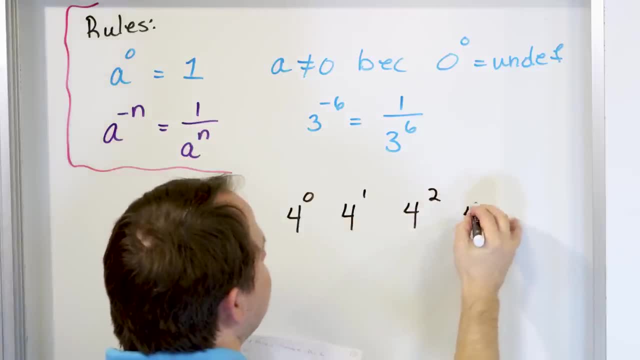 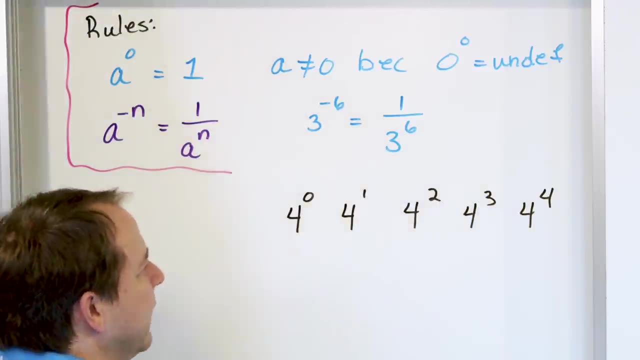 that go up like this: four to the power of one, four to the power of two, four to the power of three, four to the power of four. So here we start: four to the zero. we can increase the exponents here right, And now we haven't talked about these yet, but now we know that also on the left-hand. 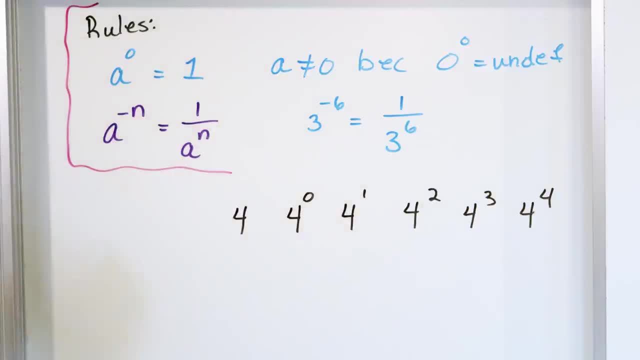 we have negative exponents because these are the positive numbers, these are the negative numbers, so we can have negative exponents. So here you might have four to the negative, one, four to the negative, two, four to the negative, three, four to the negative, four. right Now, I just told you a. 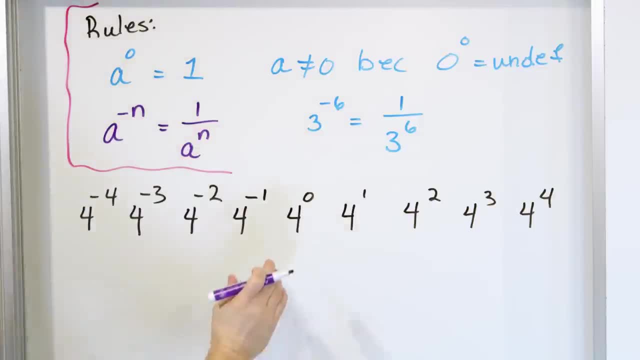 minute ago that anything to the zero power is one. but first let's just hold that in our back pocket. let's go all the way to the end When you write this. actually, let me back up for a second. let's write it like this: Let's write these over here: four to the zero, four to the one. 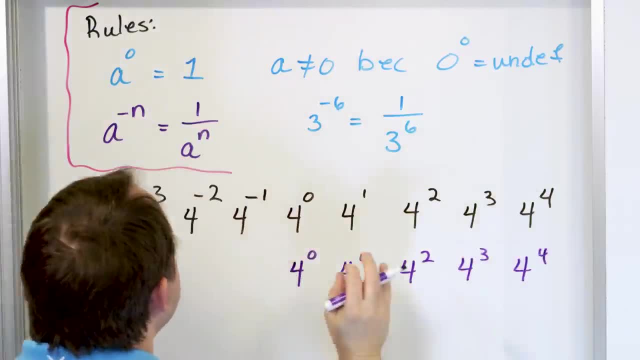 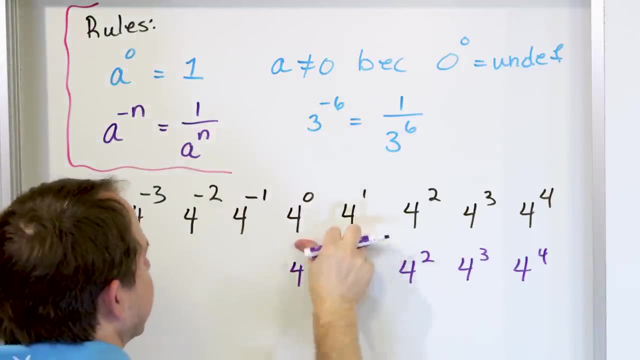 four to the two, four to the three, four to the four. According to this rule here, this one which I haven't used yet, let me erase this one According to this rule here that I haven't used yet, but we're going to use it for the first time- four to the zero, power is one, And according to 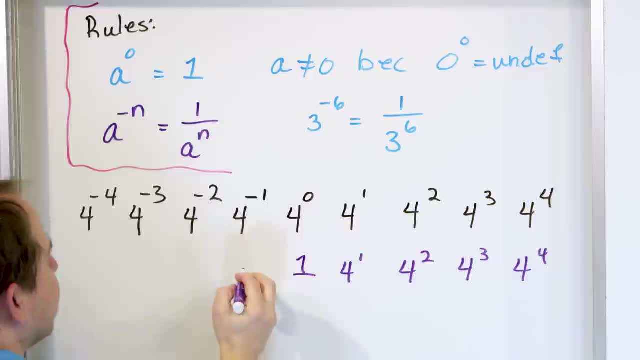 this rule, which we haven't used yet, but we'll use it now. this guy is really equal to one over four to the first power, And this guy is really one over four to the second power. And this guy is one over four to the second power, And this guy is really one over four to the second power. 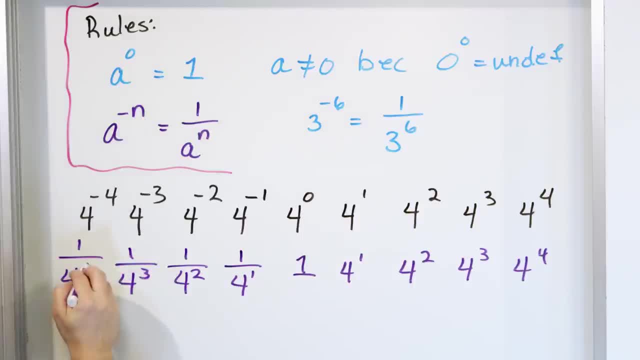 to the third power, and this guy is one over four to the fourth power. So you see how the pattern goes. You have exponents that are whole numbers, and then again the exponents are whole numbers here, but they're in the bottom of the fractions. So why am I doing this? you say Because, as you 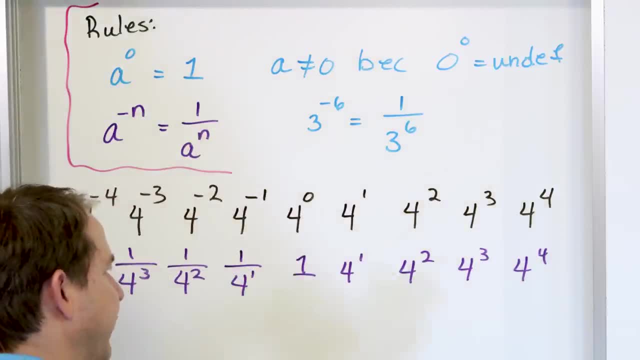 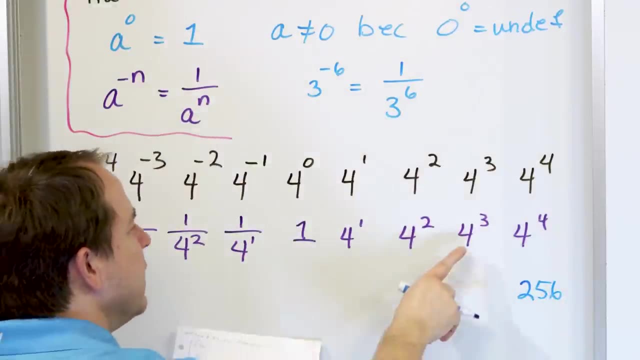 can see- let's start off on the right hand side. What is four to the fourth power? That's four times four times four times four, right? which means that this is going to be 256.. You can verify that in a calculator. Four times four times four is four to the third, that's 64.. Four squared, you all. 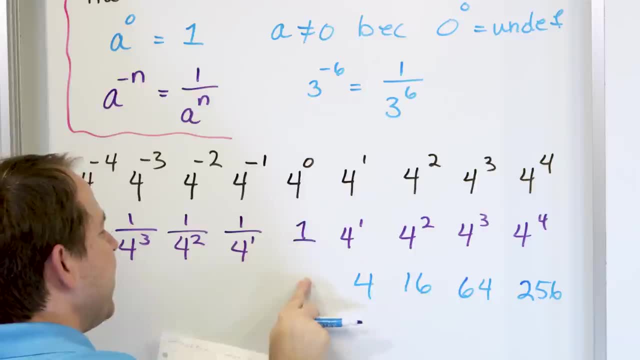 know, is 16.. Four to the first, you all know, is four. Then we have this number one which lives in the middle. Now, if four to the first is four, then one over four to the first is one fourth. That's what's this here. And if four squared is 16, then one over four squared is one over 16.. And by similarity, 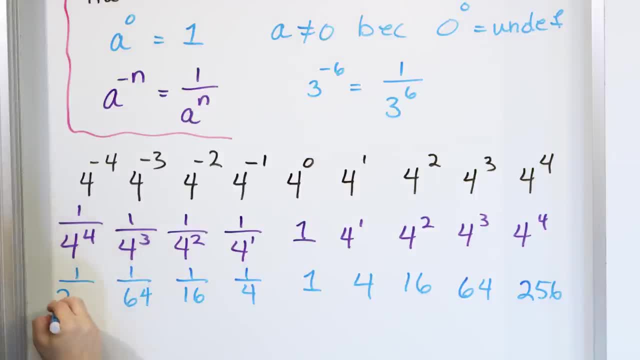 this is one over 64 and this is one over 256.. Why am I writing all this stuff out for you? It's because I want you to see that kind of in the middle here we have the zero power. That's the middle here, which means it evaluates to one. I haven't proved it to you yet. 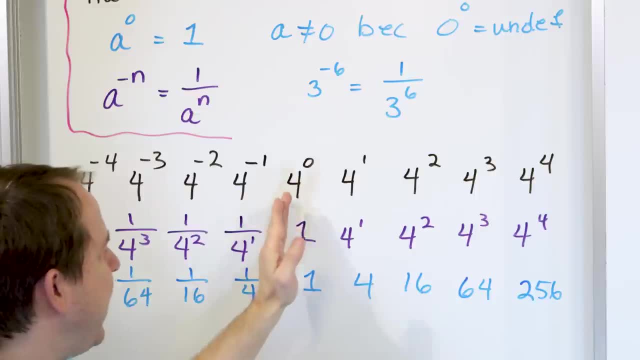 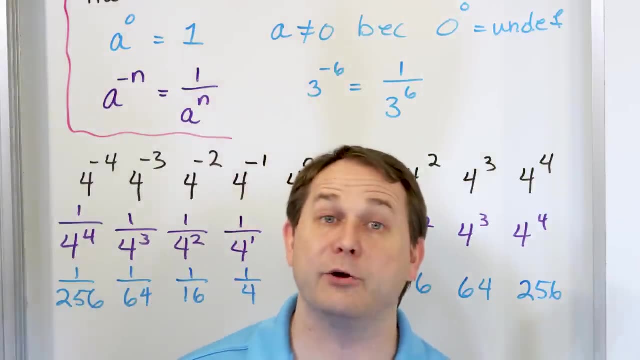 but anything to the zero is one. As you take your base and have positive exponents getting larger and larger, the value of the thing you have is getting bigger and bigger because the exponent's getting bigger Makes sense. But then as you start from your neutral point again and go the other, 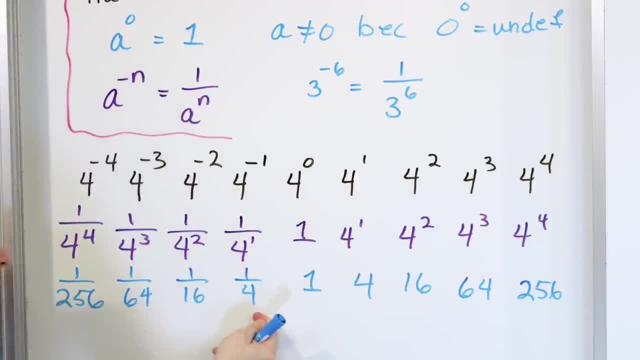 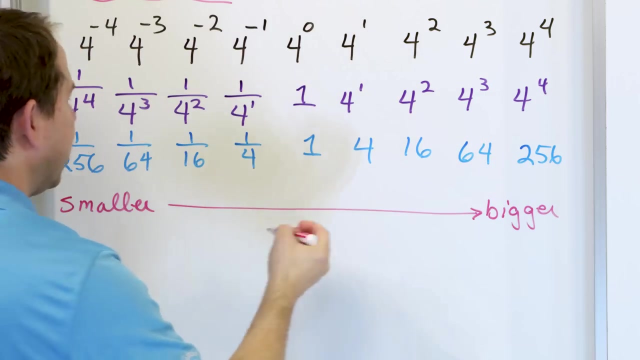 directions. the numbers get smaller and smaller, because one fourth is bigger than one, sixteenth is bigger than one, sixty-fourth is bigger than one, two, fifty-six. These are really small numbers and these are larger fractions, and then these are even larger whole numbers. So really, what you have is you have smaller going to bigger. Why am I doing all? 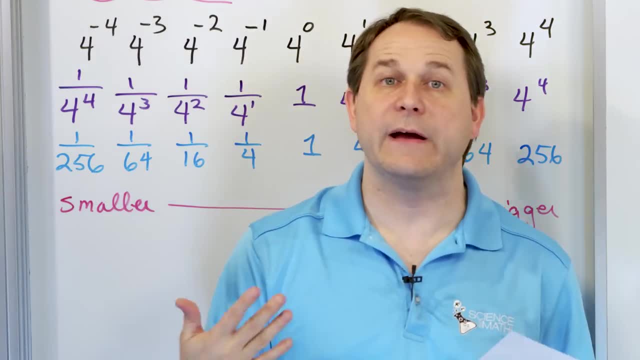 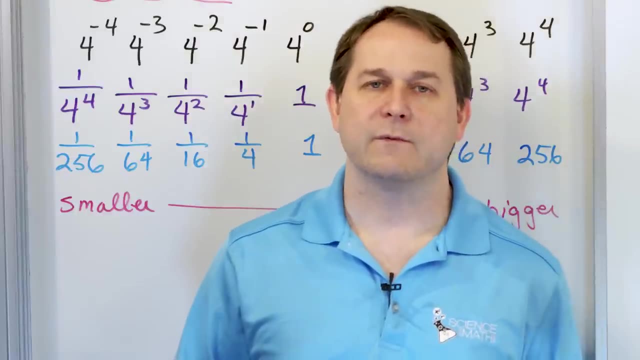 this I want you to get in the back of your mind: that when you have negative exponents, it means that it lives on the bottom of the fraction, which means the value of whatever it is is a small number. When you have fifteen to the negative twenty power, that's a small number, not a big. 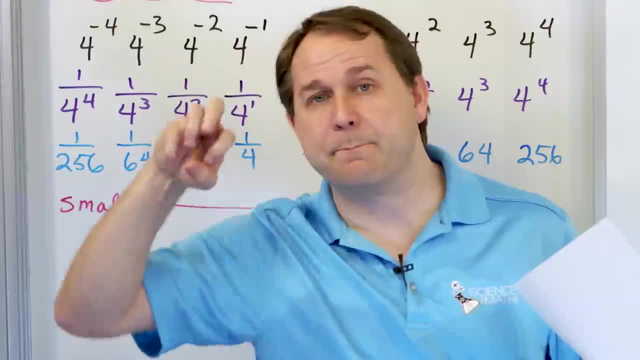 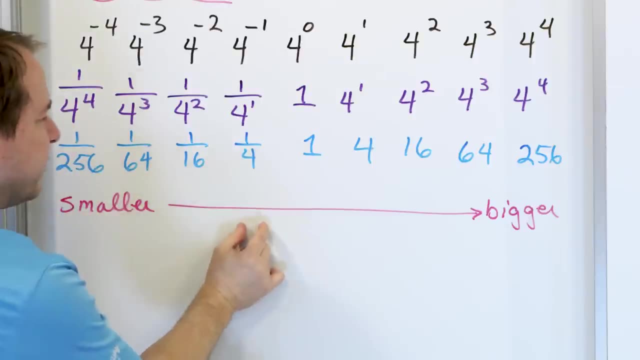 number. A lot of people think, oh, the twenty power is huge, but the negative means it's on the bottom of a fraction. So, just like this guy was on the bottom of a fraction, it means this is really, really small. This is a small decimal. This is also a decimal point two, five, but it's much bigger. 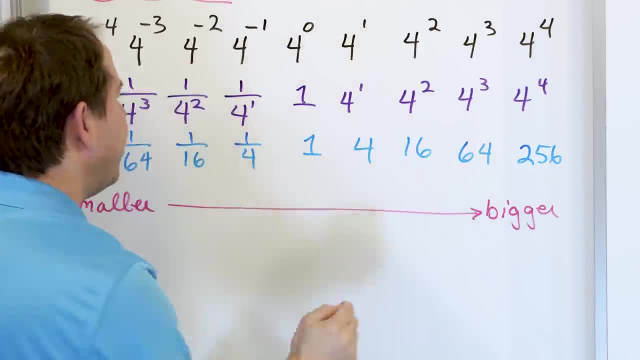 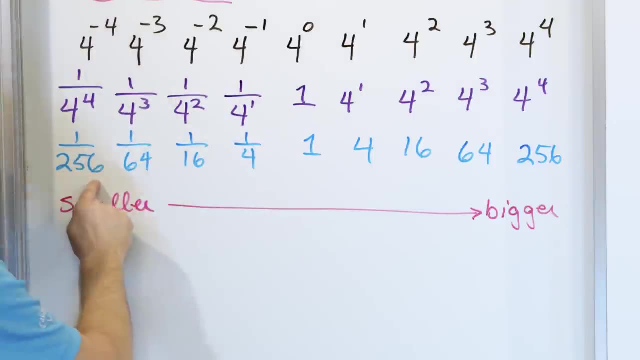 Then we have one which is neutral in the middle and then it gets larger from there. So the negative exponents, when you get negative large exponents negatively, you have really really small numbers as you get to the zero power, which is the neutral point one, increasing even more, getting larger. 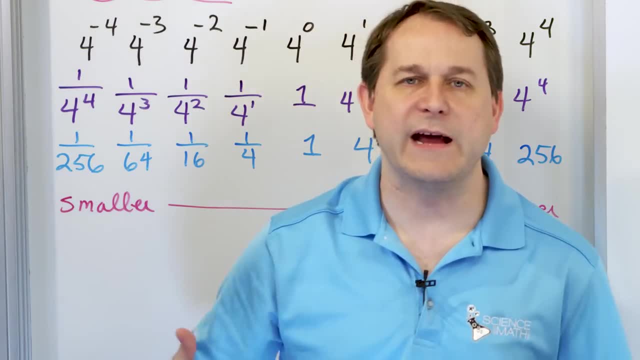 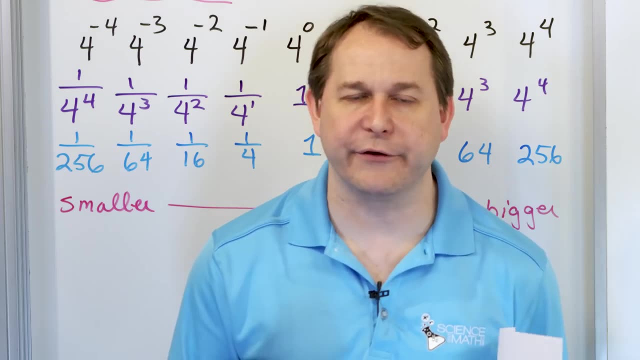 So the whole scale of it is smaller to bigger. frequently In science we talk about- we'll talk about later- scientific notation. You know, atoms might be ten to the minus ten meters. The minus ten meters. That means a really small number, Whereas galaxies might be really far away. ten to 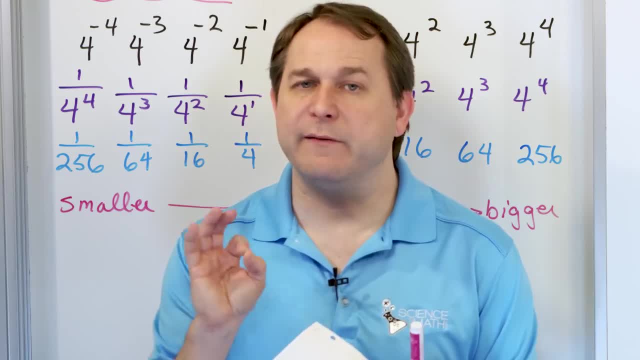 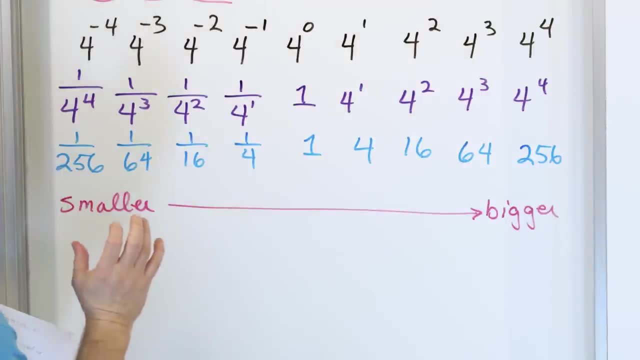 the twenty, whatever unit it is. So negative exponents means small numbers, Positive exponents mean large numbers. I want you to get that in your head Now. I want to turn my attention next to showing you why this is true. Why is it that anything to the zero power is one, Of course, except zero raised to the zero power? 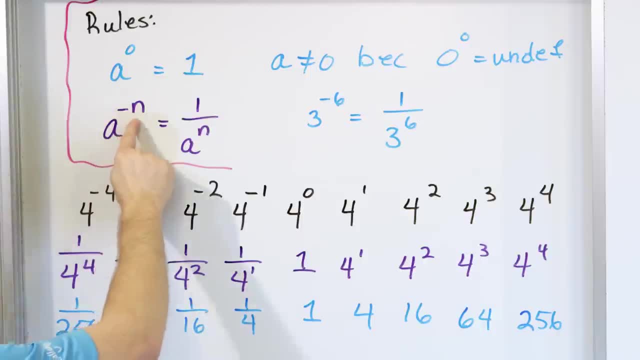 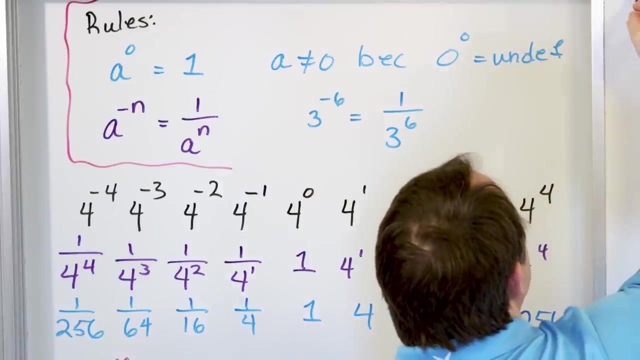 That's undefined. And why is it that anything raised to a negative exponent is just a fraction, with the exponent turned positive and brought into the denominator? I want to go over why those rules actually work. So let's take them one at a time. Let's talk about this first one first. So we'll say: 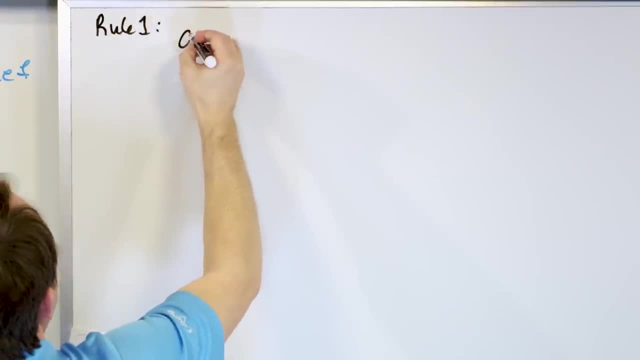 rule one, which is what A to the zero is equal to one. So let's start in math. when you do a proof like this, Usually what you do you start with something you know is true, And we know that a base to an nth exponent times a base to the nth exponent. 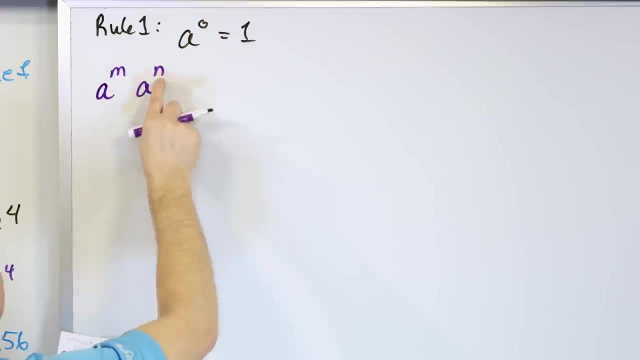 These are different numbers, like it can be A squared A to the third. What do you do If the basis of the same, the exponents, are different? you add them right, so it's A to the m plus n. this is exactly like A squared A to the third. you add them: two plus three is five. 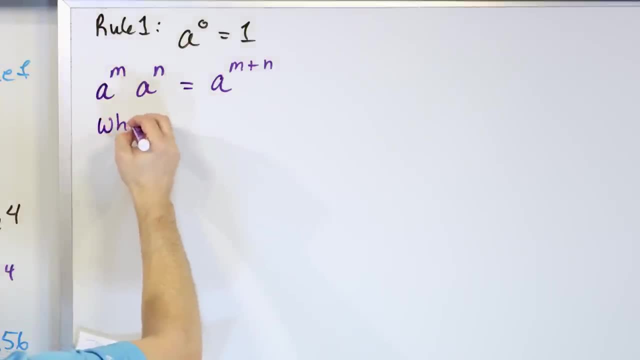 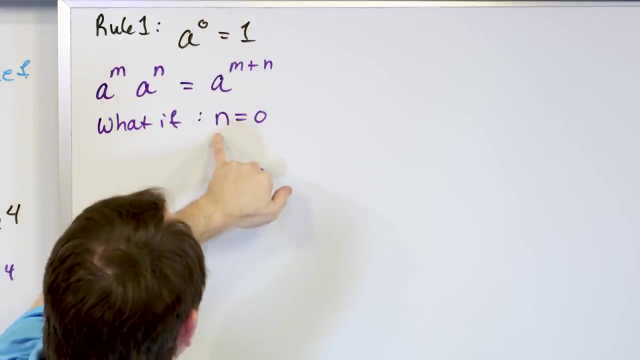 the exponents. But what if? what if n was equal to zero? In other words, we're trying to show that what if an exponent is zero? Let's set one of these exponents equal to zero and see what actually happens Then in that case. 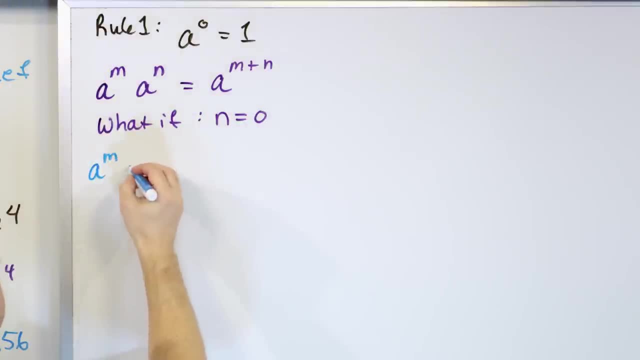 what we would have on the left side here. we would have a to the m, but let's set n equal to zero. Then on the right hand side, we have a to the m plus zero. So all we're saying is: we know this is true. we've been using exponent addition. 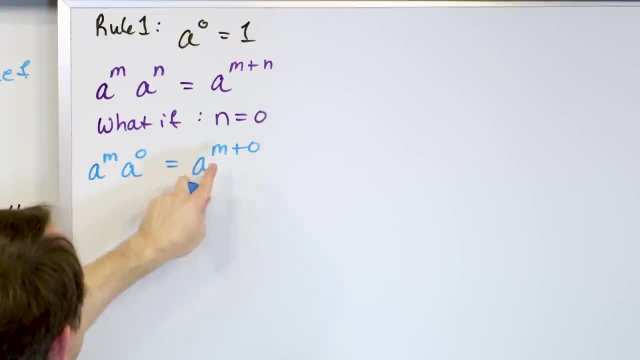 forever. let's set one of the exponents to zero. That means that it's going to be one of them. set to zero. add it up here. So what do we have in the next step? It'll be a to the m times a to the zero equals. well, what happens when you add? 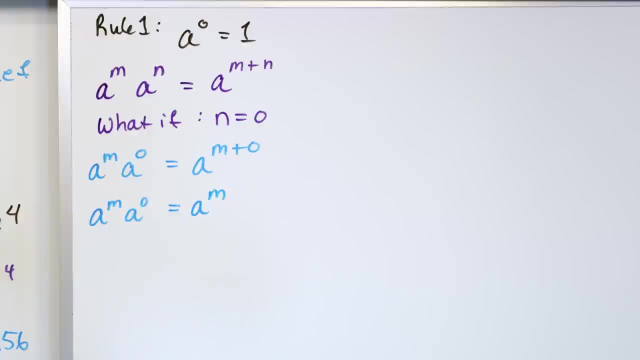 zero to something. Just going to get a to the m back again. okay, Now we want to figure out and prove that this is equal to one. So how do we isolate it? We're going to divide both sides by a to the zero power. So you have a to the m. 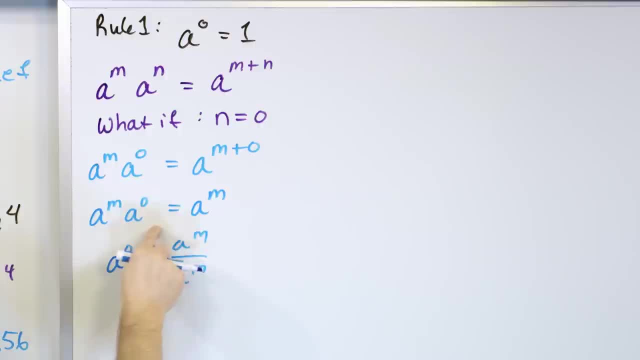 a to the m. What do we do? We took this equation. we divide by a to the m. that kills it on the left. Divide this by a to the m and you can see that what you're going to have this is the same on the top and the bottom. so they cancel, or you. 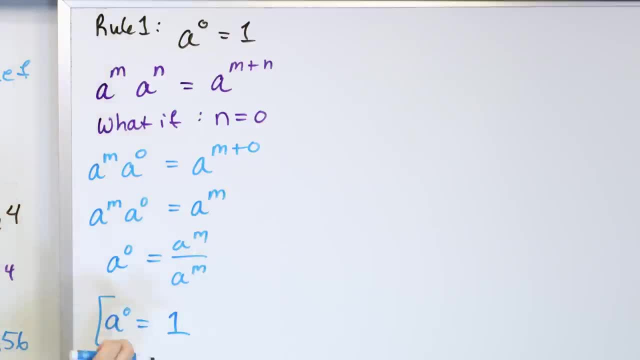 can think of them as dividing and always giving you one. So we've proven that any variable raised to a zero power is one. Any number raised to the zero power is one. Now, if you go back to the original rule that we had, we said that this was: 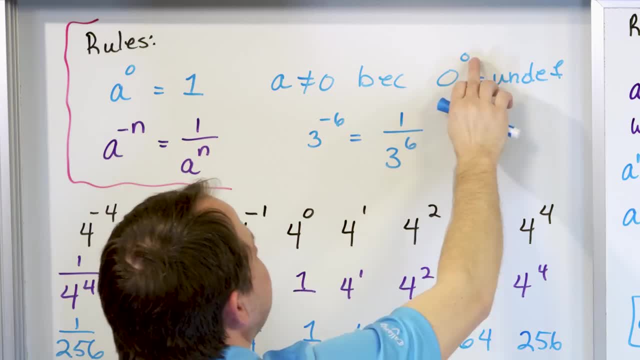 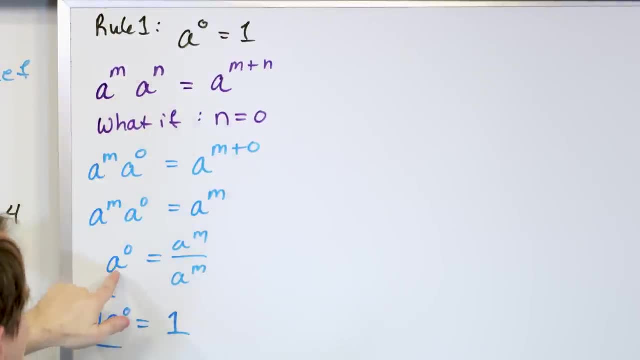 true, but only if a was not zero. We said that zero to the zero is undefined. It doesn't exist. Now, from the proof, we can see why: Because if we allow a to actually be zero, so it's zero to the zero power, then that would mean you would have zero to the m, zero to the 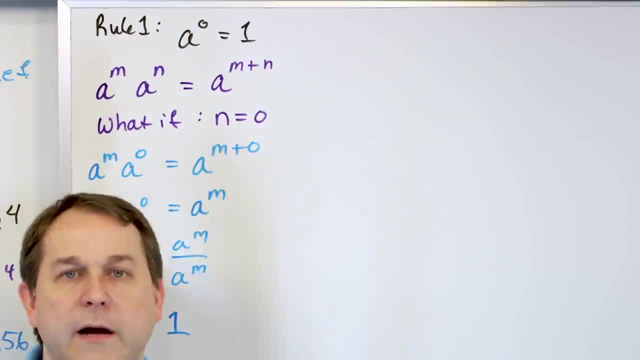 m right, But on the bottom, cover up the top. zero raised to any power, Zero raised to any power is going to give you zero. Zero squared is zero, because you know zero times zero, right, It gives you zero. Zero raised to any power gives you zero. 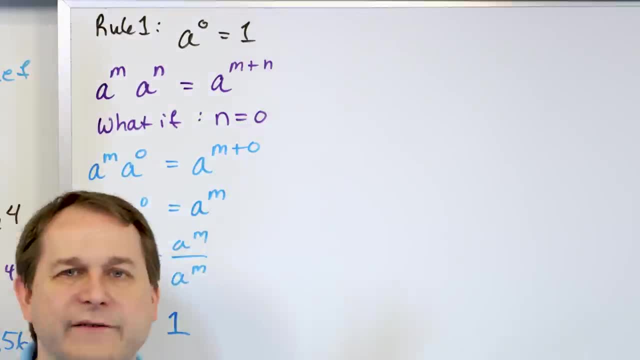 right. So if I have a zero in the denominator of this fraction, I can't divide by zero. I mean in calculus we say it approaches infinity or something, but in real life you can't actually divide something by nothing. You get an undefined. 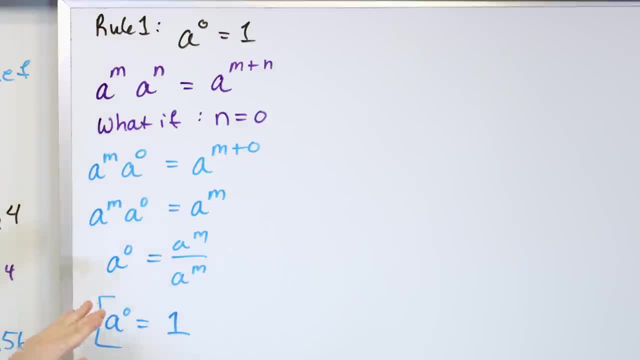 nonsensical answer. So because we can't do that, we exclude the possibility when a is actually zero and so we say zero raised to the zero is not defined because you get, you have problems actually pulling this off. But for any other value of this? 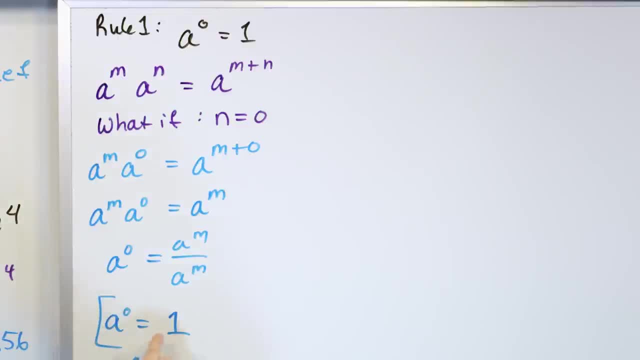 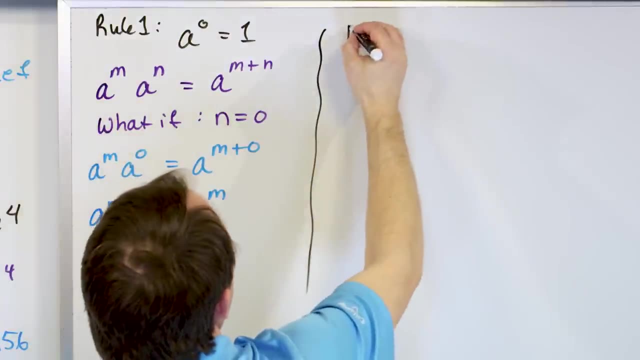 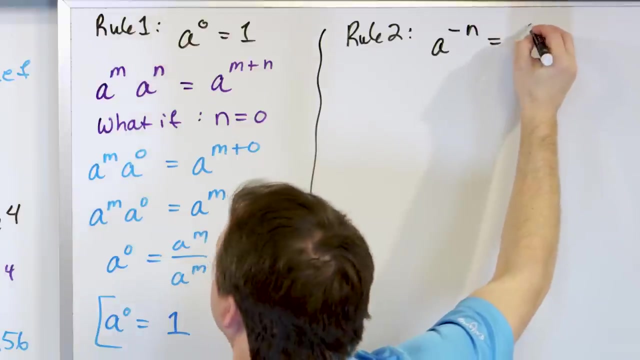 variable a. when you raise it to the zero, 0 power, you always get 1,. all right, So that's where it comes from. Now let's talk about rule number two. So rule two is almost more important, really. a to the negative n is equal to 1 over a. 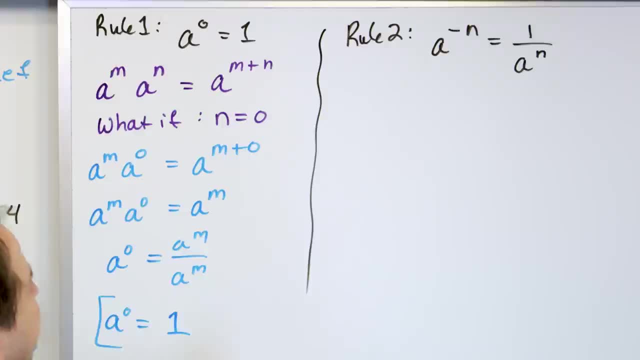 to the n. This is the one you're going to use constantly when you're solving problems. When you see a negative exponent, you just make it a positive exponent by pulling it downstairs. Why is that true? It seems like magic, right? Well, let's go back and start with what we know, And 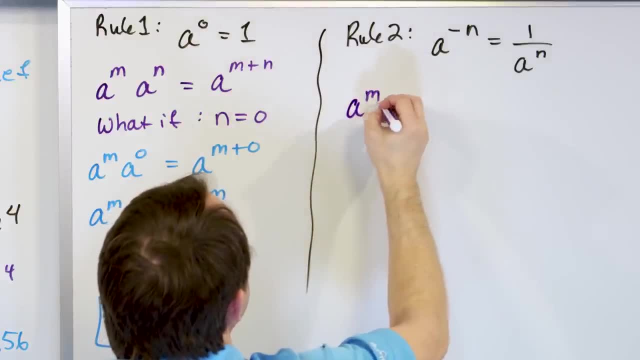 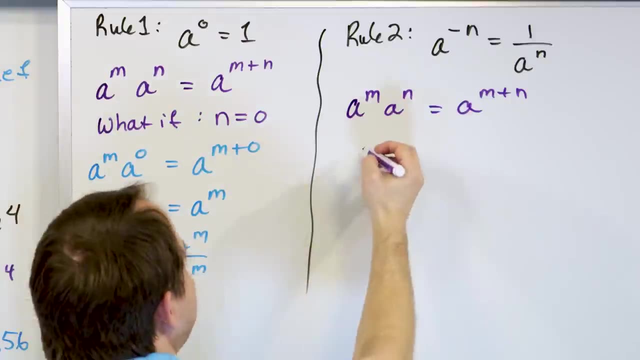 we know we're going to start from exactly the same point as the other guy: a to the m, a to the n. we just add these exponents, m plus n, just like we did there, no difference. But now let's say: 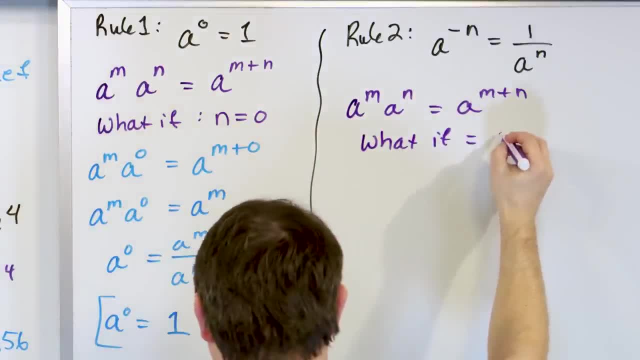 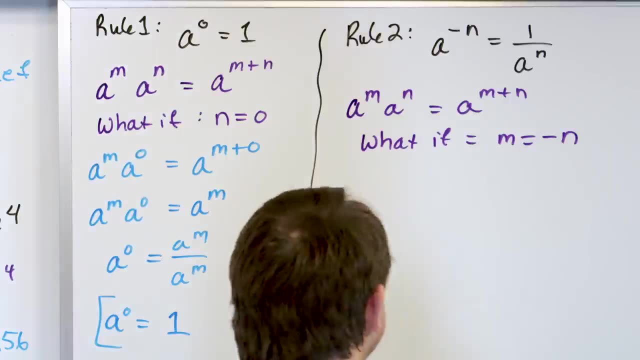 what if one of these exponents, m, is actually equal to negative n? In other words, we want to set one equal to negative n, so we'll make one of these exponents equal to negative n. What's going to happen when we make that substitution? So if this is negative n, it'll be a to the 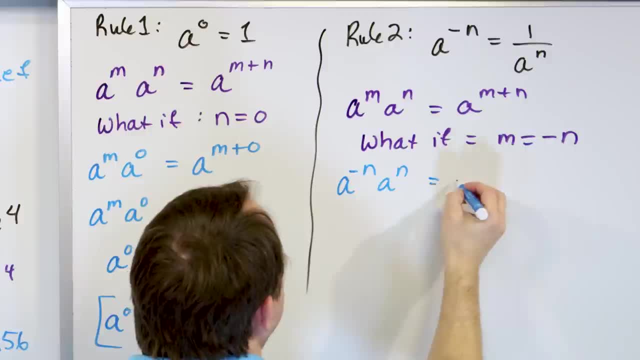 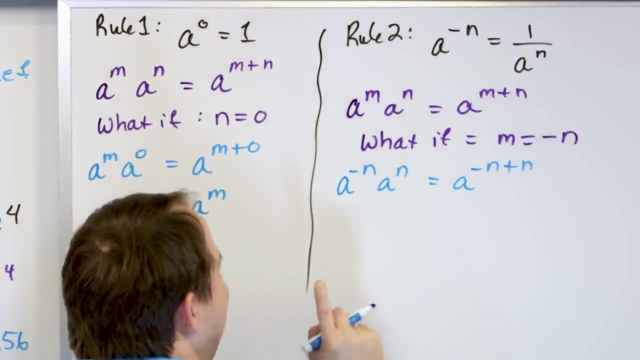 negative n times a to the positive n. So a to the n equals a. what do you have here? Negative n plus n. All we did was make the substitution and put it in there. Now what's going to happen is when you add negative n to n. 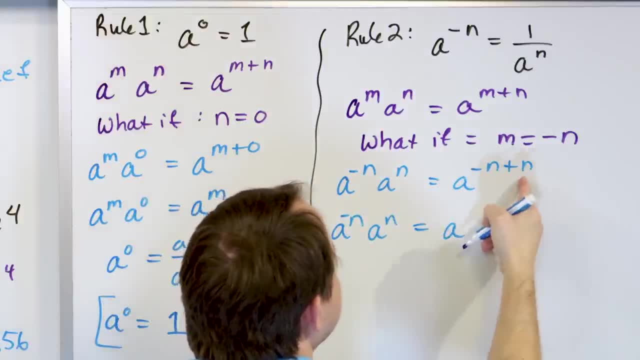 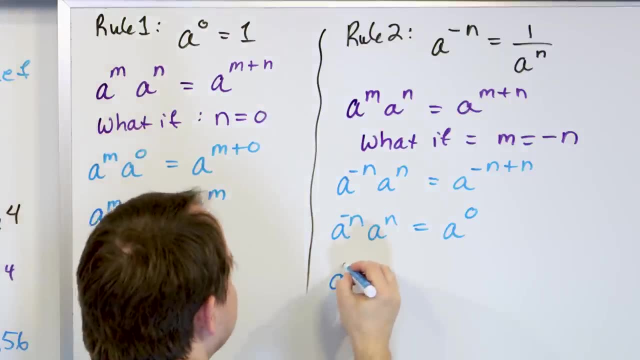 a to the n equals what are you going to have? A to the negative n plus n is a to the 0. But you already know that a to the 0 is 1.. So what you really have is a to the negative n. 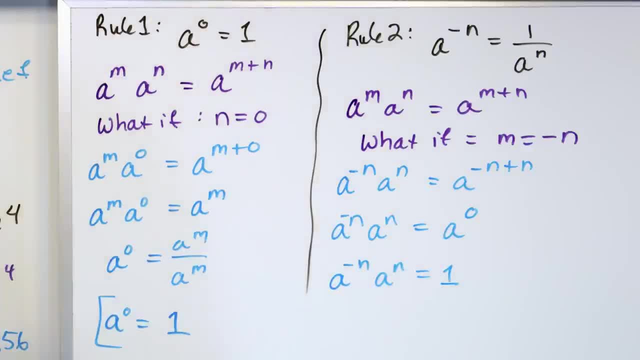 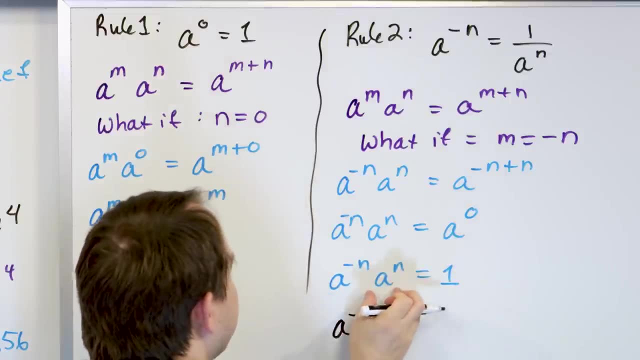 times a to the n is equal to 1.. So now we're trying to prove to ourselves what happens when you have a negative exponent. What you're going to have is divide both sides of this equation by a to the n and you're. 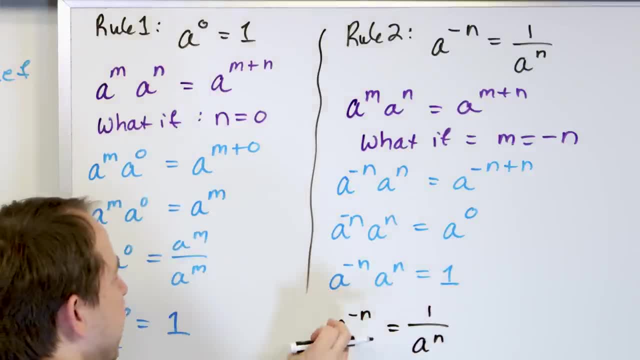 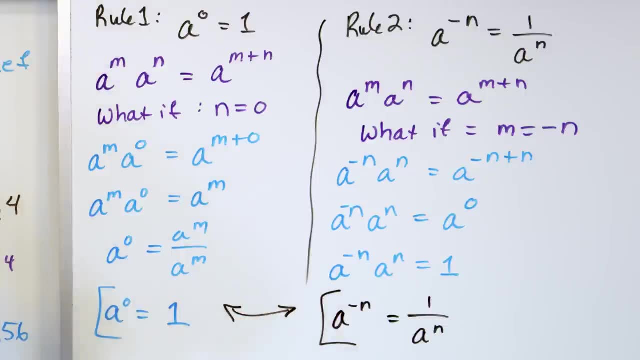 going to get 1 over a to the n. Divide the left side by a to the n. canceling divide the right side by a to the n gives you this: That's the final answer. So these are the two rules that we set out. to prove And notice that all we did to get those rules is we start. 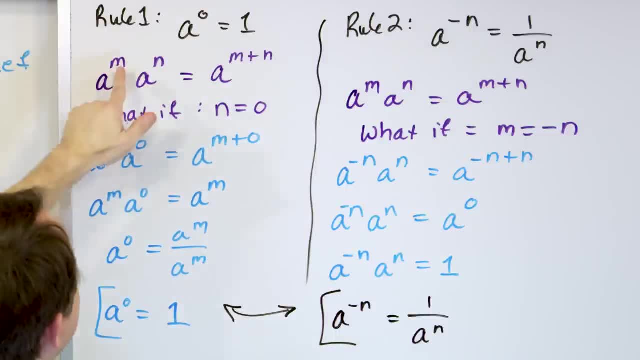 with exponent addition. We know that we have the same base, different exponents. we add the exponents. We started from the same place in both cases. This case we said let's let one of these exponents equal 0. In this case we said let's let one of these exponents equal a negative number, And then 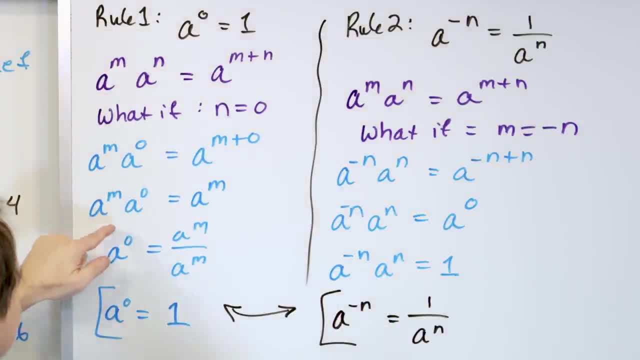 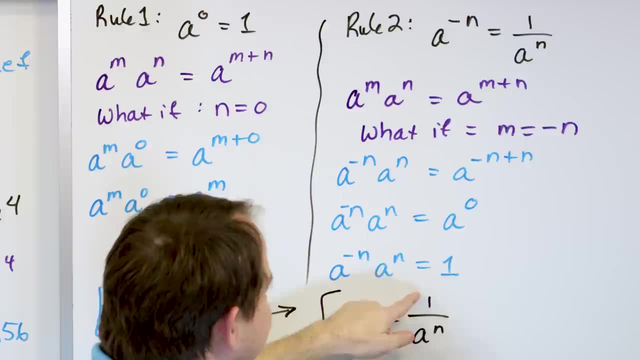 we just flow through it and we find out that when you raise anything to the 0 power, you always get 1.. And here, when you raise anything to the negative exponent, negative n, it's the same as the reciprocal of that positive exponent, 1 over a to the positive version. 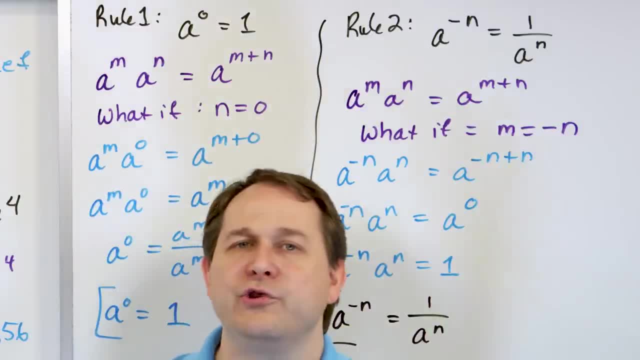 of that same exponent. That's where they come from. Will you need to use these proofs in real life? No, probably, unless you become a mathematician. But we do need to use the results all the time, Because in equations very often you'll have an exponent or something raised to the 0 power. 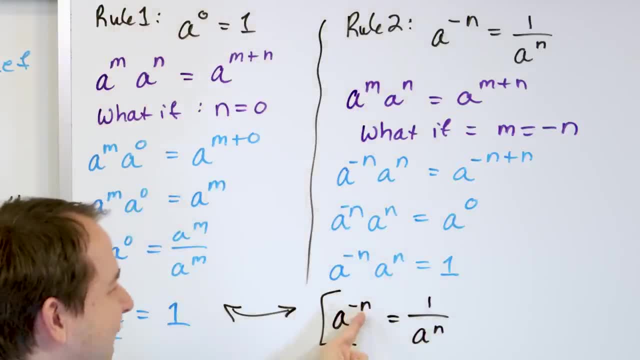 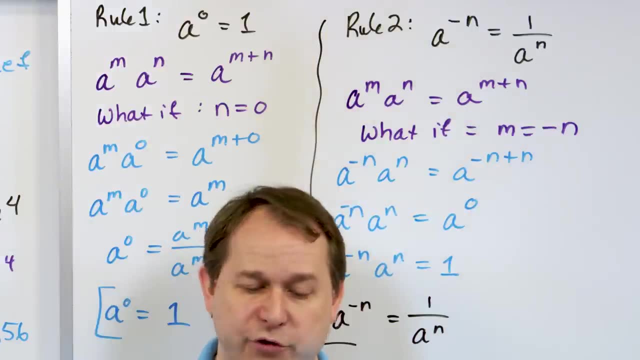 And even more common than that, we will have some expression raised to a negative exponent, which means you'll have to write it basically as a fraction, to simplify anything. So now that we have all that underway, I would like to give you a few kind of easier problems. 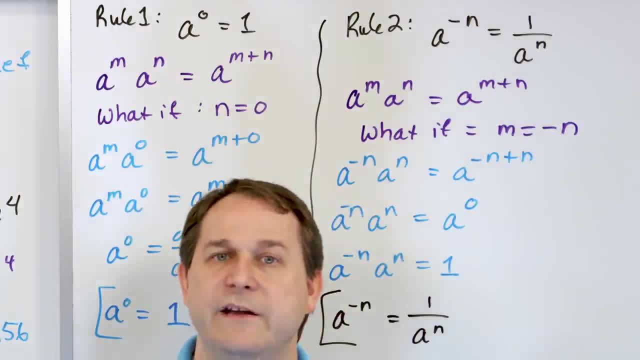 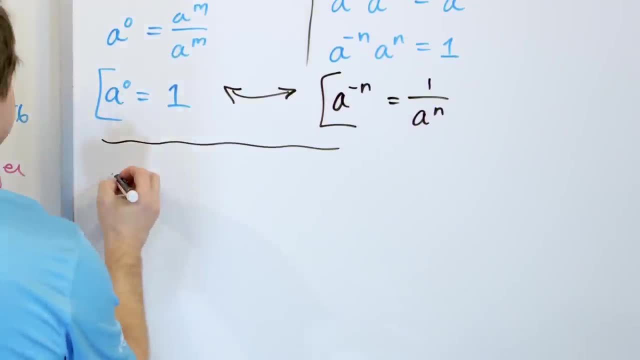 first one on this board right here. What if we have very simple start kind of basic problem? what if we have 3 times 5 to the negative 1?? We cannot add these exponents because we have different bases. But what we do know is that when you have a negative 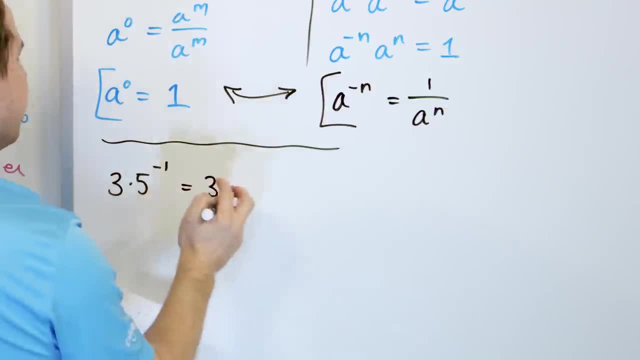 exponent. we write it as a fraction, So this is going to be three times. This is going to be written as: what did we say? 1 over the positive version of that exponent, 1 over the positive version of that exponent, which was negative: 1, now becoming positive: 1 once. 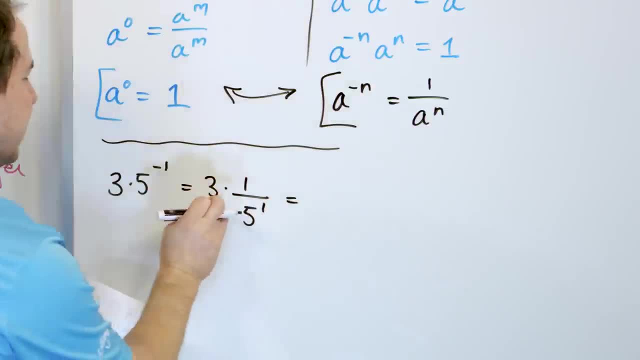 we move them downstairs, Then what do we have? If you want to be explicit, this 3 is really 3 over 1, and it's multiplied by a fraction, 1. fifth, because 5 to the 1 is 5.. 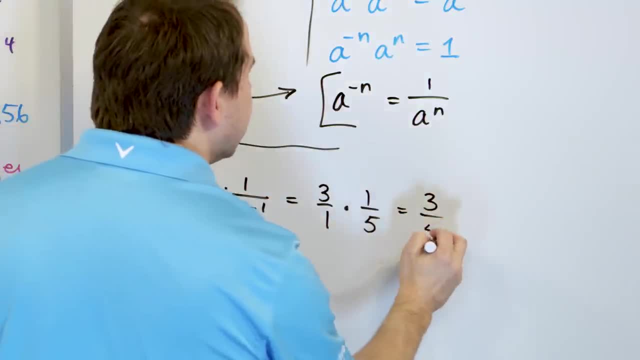 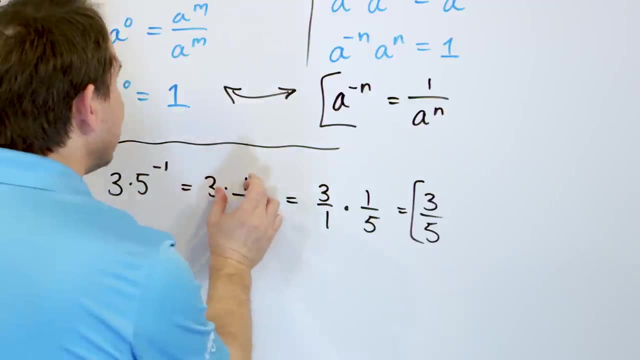 You multiply the tops 3 times. 1 is 3.. Multiply the bottoms and you get 3 fifths. All right, Three fifths And that's the answer. So when you see a negative exponent, you need to write. 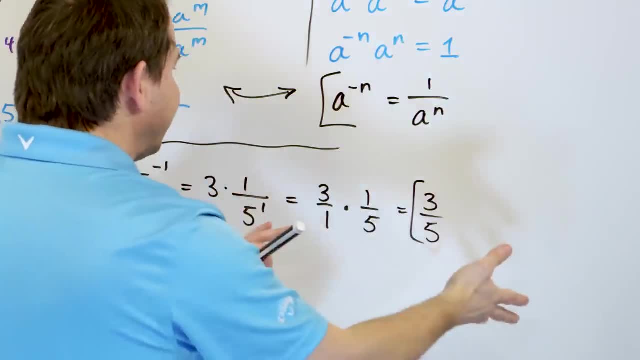 it as a positive exponent in fractional form, deal with the fractions and then get the answer. That's why I stress so much in the beginning of all of these outliers, I stress so much in the beginning of all of these outliers, I stress so much in the beginning of all of: 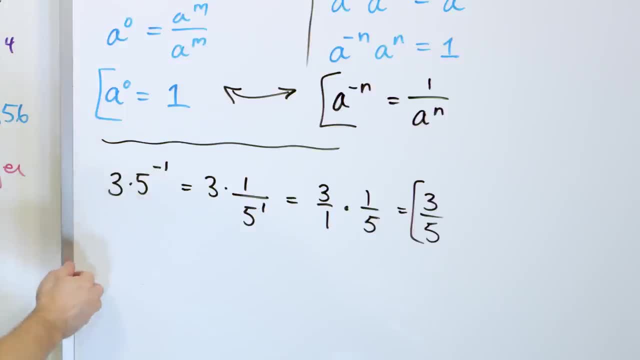 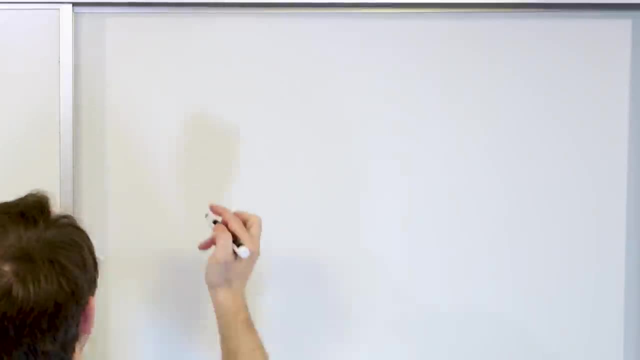 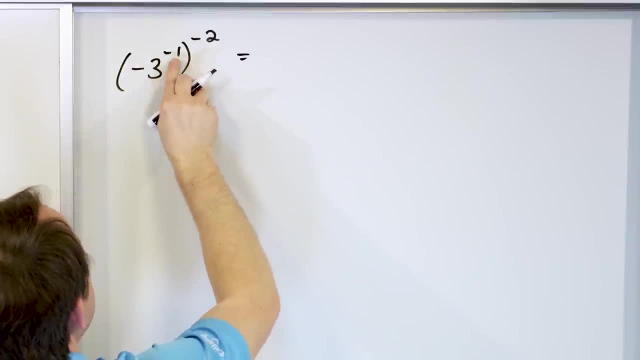 inside We have negative 3 to the first power. Now this negative 1 exponent does not apply to the negative sign here because there's no parentheses around it. If I had the whole thing wrapped in parentheses then it would apply. But when there's no parentheses, the 3 gets the. 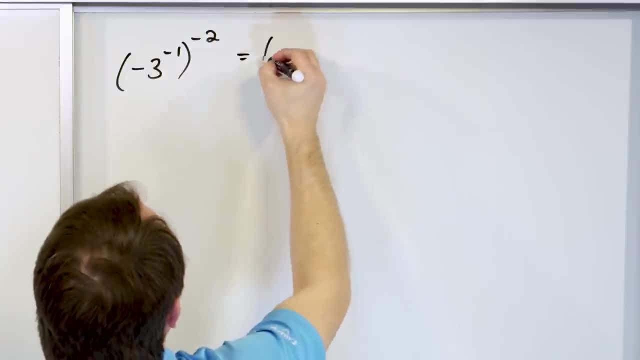 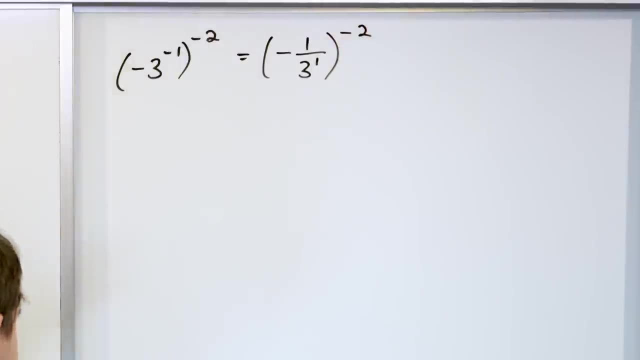 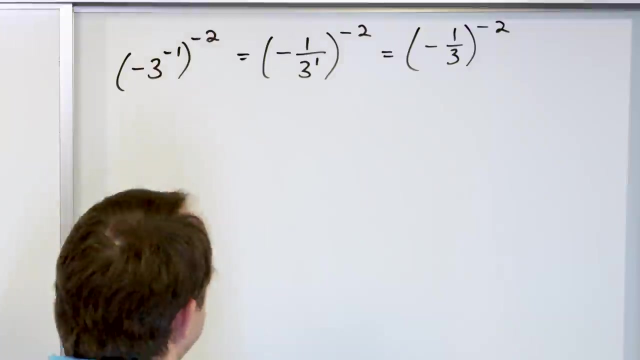 negative 1 exponent. This negative just sits outside. So what you really have on the inside is negative 1 over 3 to the first power, which is 1 third, of course, All right. So what you have is just to be 100% clear: you have negative 1 third to the negative 2.. All right Now. 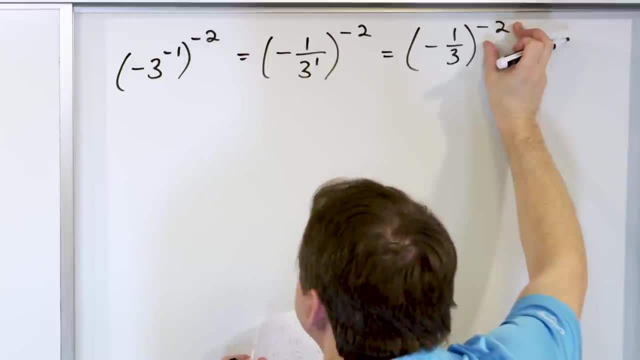 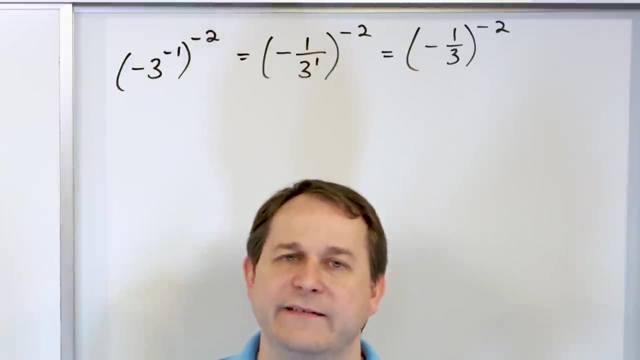 this entire thing has a negative exponent associated with it, So don't get scared by that. OK, you've got a fraction. It's raised to a negative exponent. Students are like: well, what do I do now? It's a fraction inside. It's the same rule. Whatever you have, that's. 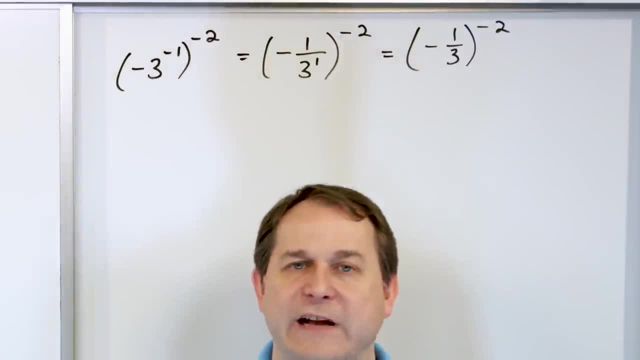 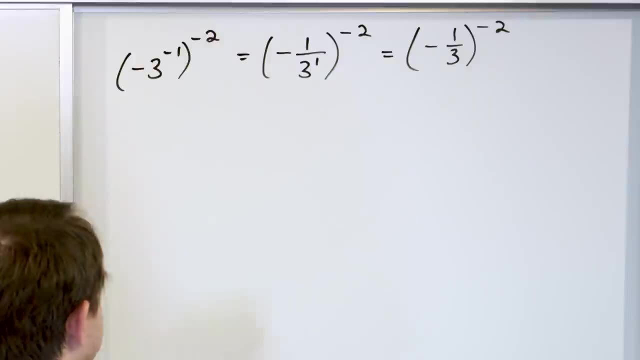 raised to a negative exponent gets moved to the bottom of a fraction, And you're just going to have to deal with the fact that sometimes your fractions are going to look ugly for a little while, But we'll do enough problem Where they won't be too bad. What we have here is what you'll have is it'll be 1 over this. 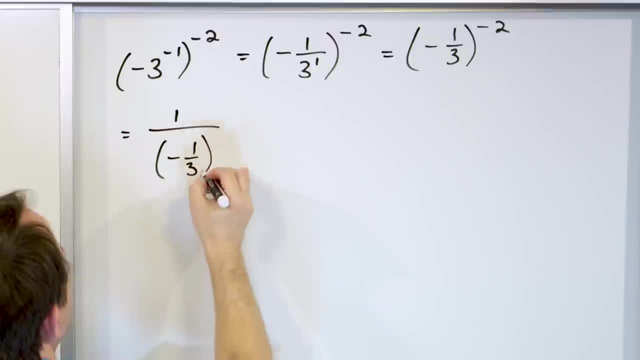 quantity here, this entire quantity, negative 1, third, raised to the power of 2.. See, I just took whatever had the negative 2 exponent, I moved it downstairs And I made it a positive exponent. Everything in the middle remained the same. Now on the top stays the same On the bottom. 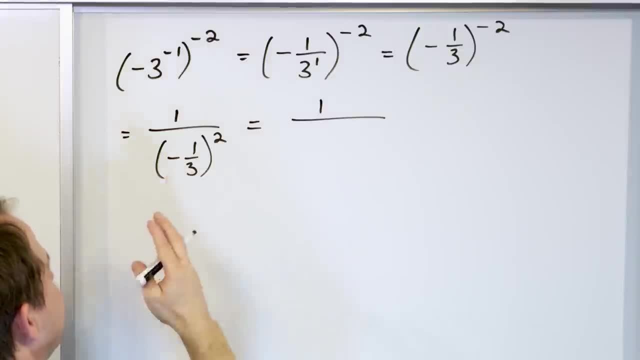 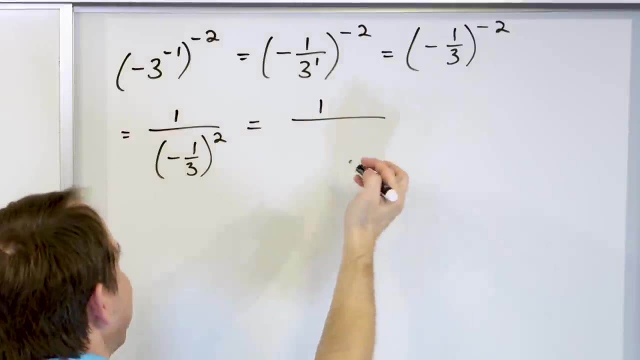 what do we have? We have negative 1 third squared, which means negative 1 third times negative. 1 third Negative. 1 third squared Negative. 1 third squared Negative. 1 third squared Negative times negative is positive And 1 third squared is 1 third times 1 third. 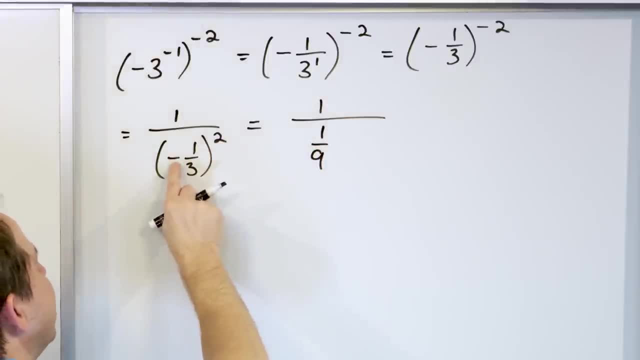 which is 1 ninth. It's positive because the square applies to this negative. So negative times, negative gives you positive And this times this gives you 1 ninth. You square the top, you square the bottom, you get 1 ninth. Now, students look at this often and have no idea. 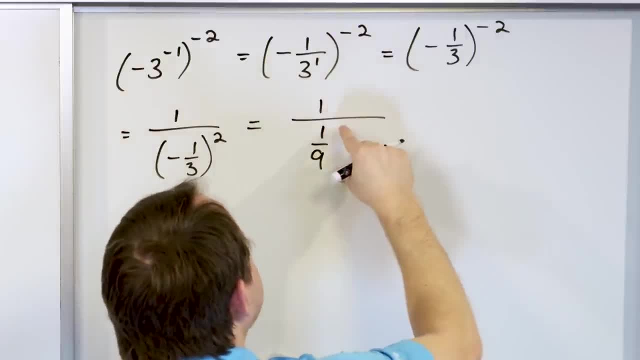 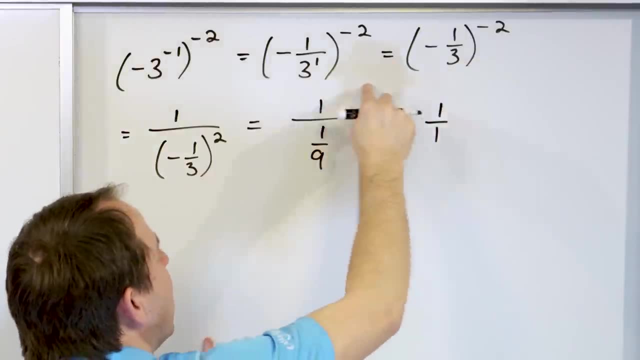 what to do. But it's just division. It's something on the top divided by something on the bottom which happens to be a fraction. So what you really have is the top here is really 1 over 1.. The number 1 can be written as 1 over 1.. 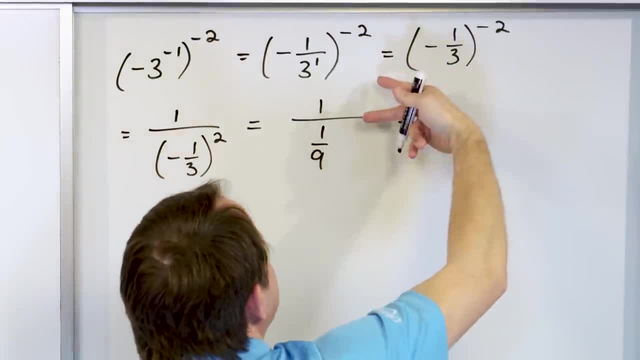 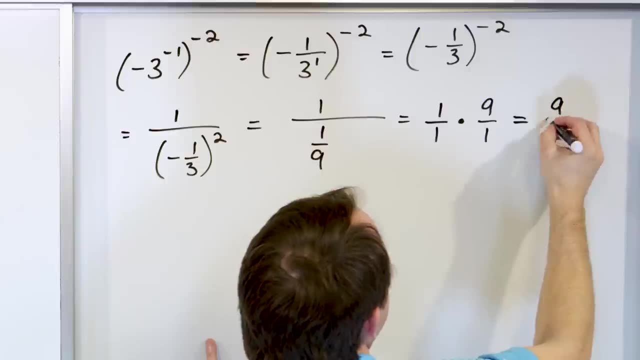 1. Change it to multiplication and take the bottom, flip it over. That's how we divide fractions: You take the bottom, flip it over, make it multiplication. What do you get? 1 times 9 is 9.. 1 times 1 is 1.. And of course you know, 9 over 1 is 9.. So the answer is just: 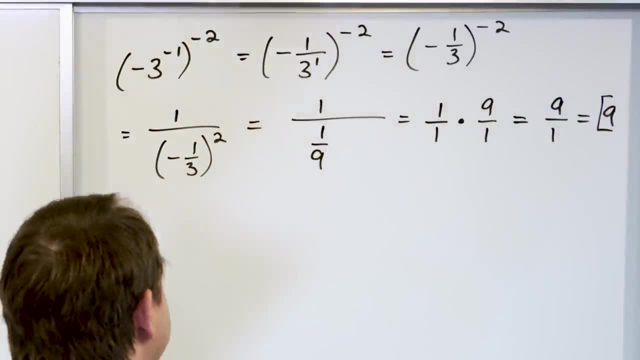 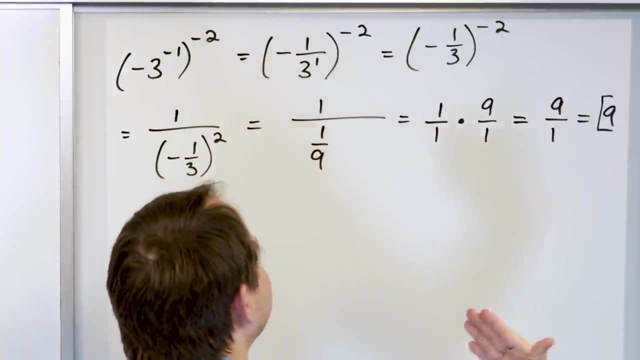 9.. A couple of things I want to point out before we go to the next problem: 1 over a fraction. I want you to do it like this, But in general, after a while you'll start realizing when you have 1 over a fraction it basically just means you take the reciprocal And that's. 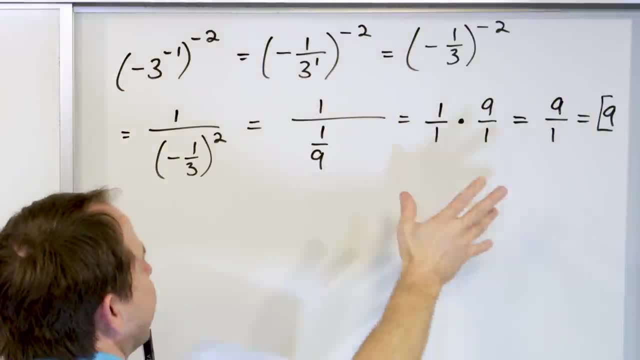 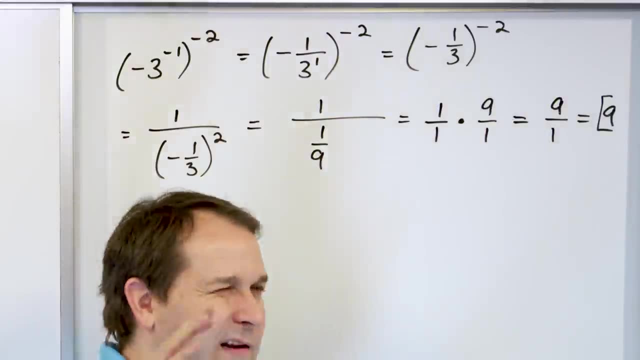 the answer. So the reciprocal of 1 ninth is 9.. I'm showing all the multiplication to make it clear what's happening. You're dividing something, you change it into multiplication and that gives you 9.. But when you start seeing lots of fractions on the denominators of larger fractions, you'll 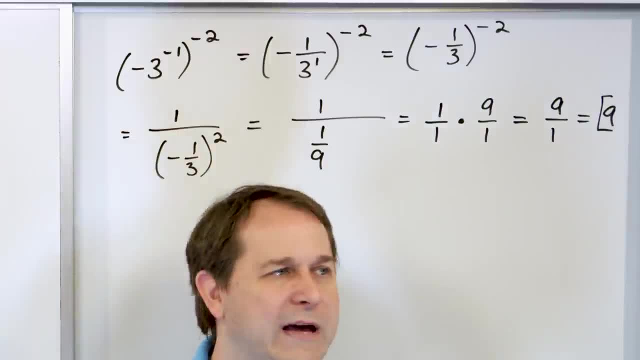 realize you can kind of flip them over, because that's what's happening. We can kind of think of this 1 ninth as being like a trapeze artist. He's kind of hanging. He can swing up and flip himself upside down to the top. That helps you, Whatever. Everybody does things differently, But that's. 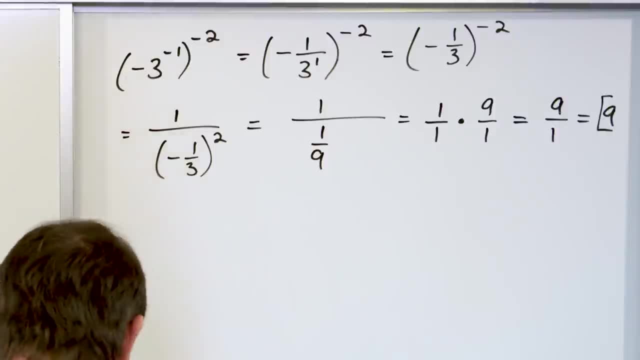 what's going on here? This division becomes a multiplication. You flip it. Now I do think it's very, very important for you to understand different ways of doing things. So I want to take this problem and do it again differently. Negative 3. And I 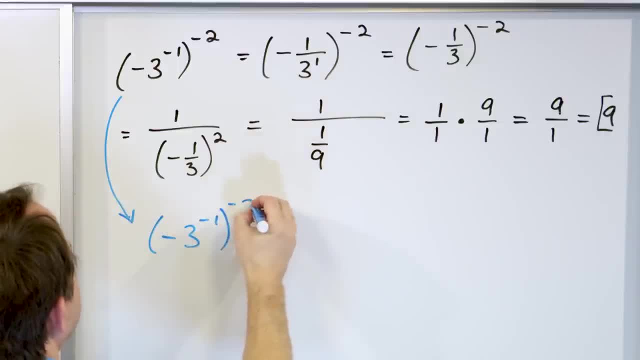 don't even have this in my notes, So hopefully I don't fumble too much, But I think it's important What we have here. remember I told you a long time ago what if we had. before we tackle this. 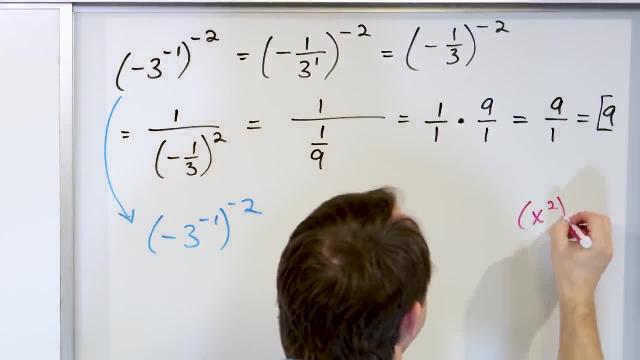 let's go over here. What if you had x squared and it was raised to the fourth power? It's a power raised to a power, right. It would be x to the eighth. It would be x to the eighth. It would be. 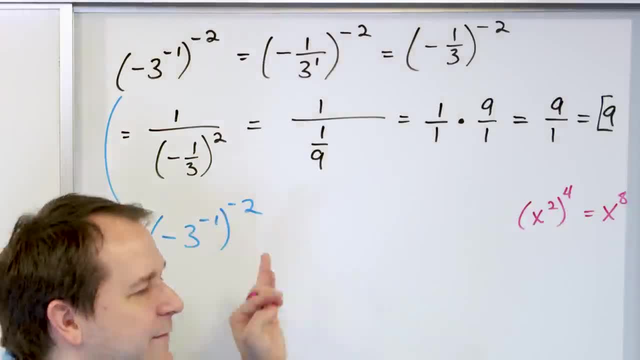 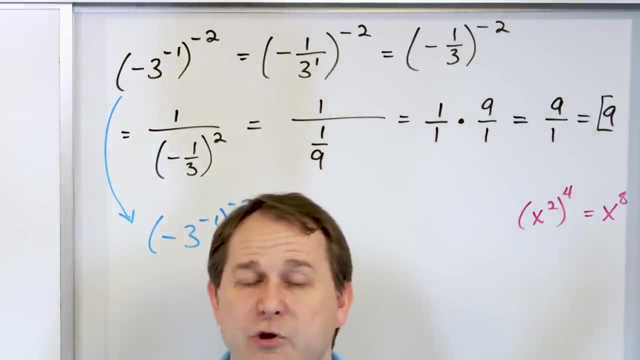 eighth, because you multiply those powers, Just because this is a negative exponent doesn't mean that it has different rules. If you have an exponent raised to an exponent and one of those exponents, or even both of them, are negative, that's okay. You still multiply them, just like. 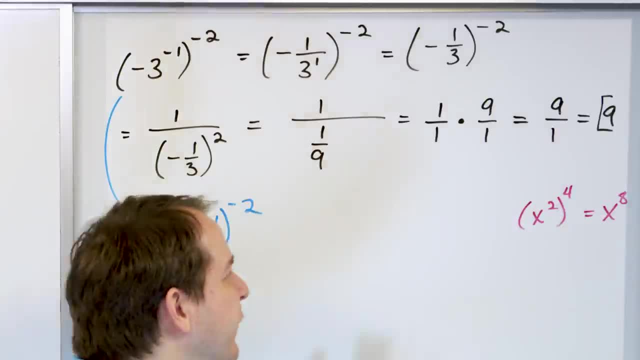 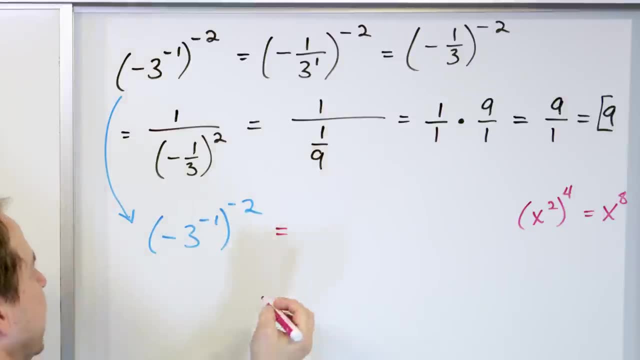 you do with regular old exponents. It's just a negative exponent. So what this means here is that I'm going to have this negative 2.. It's going to apply to everything inside. So the best way to do it is for you to realize that it's like this Negative 1, which is what's in front of here. 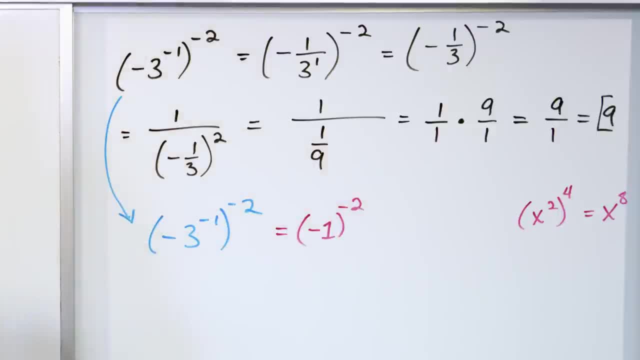 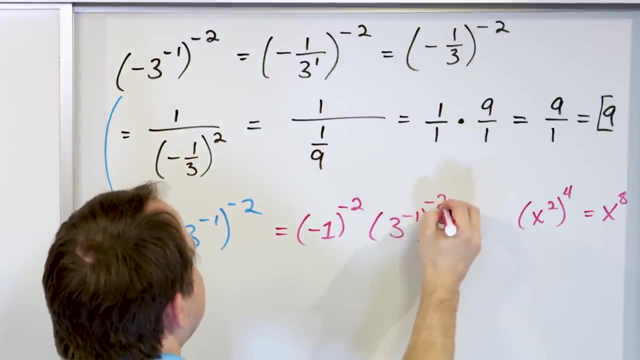 this negative 1, is going to be raised to the negative 2 power, okay, And then this guy here, 3 to the negative 1, is also going to be multiplied or raised to the negative 2 power. So this power 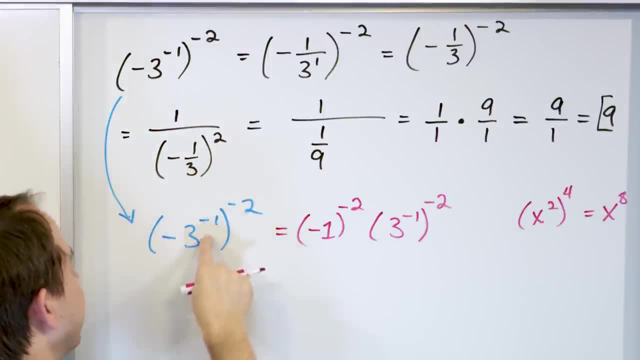 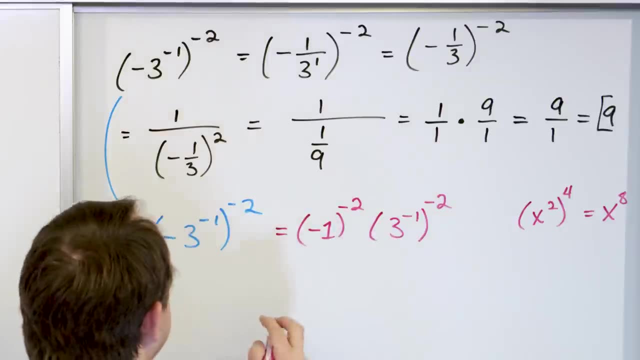 gets applied to this number, which is negative 1, also to this, which is itself an exponent, which is kind of weird. Let's go down and proceed. What's going to happen here? Negative 1 to the negative 2.. What's going to happen is it'll be 1 over whatever. this is negative 1, and we make 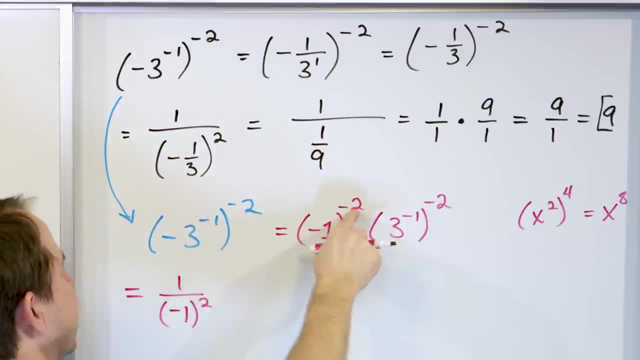 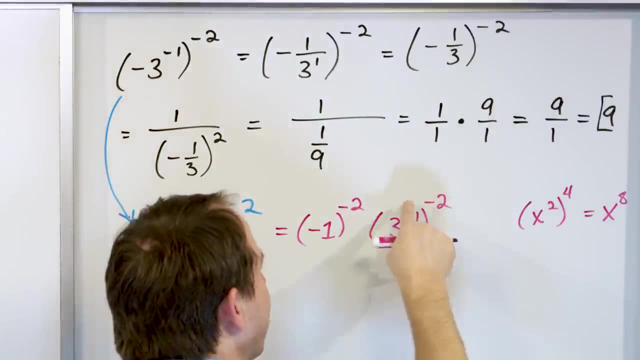 positive square. We take it, move it to the bottom, make it a positive exponent, because that's what we do. We move them downstairs. That's going to be multiplied by Now. you can do it different ways. You can make this one-third and square, but I want to show you different ways of. 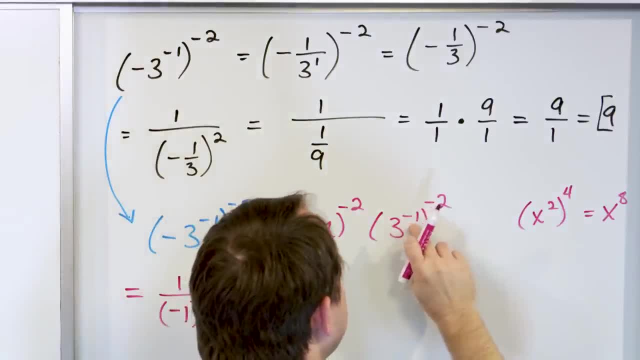 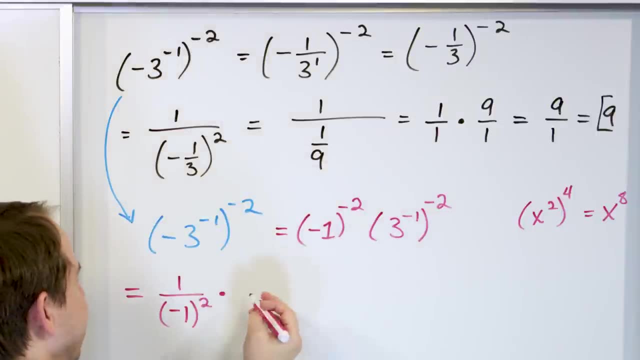 doing things. You can say the negative 1 times negative 2, because it's a power raised to a power, just like this is. So negative 1 times negative 2 gives you what Positive 2.. So 3 squared, right. So what am I going to have On the top? I'm going to have 3 squared. 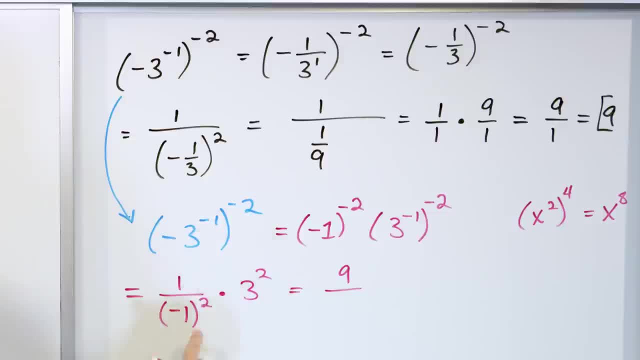 which is 9.. On the bottom, I'm going to have negative 1 squared. What's negative 1 squared? It's positive 1.. And the answer I get is 9, exactly as what I got before. So there's lots. 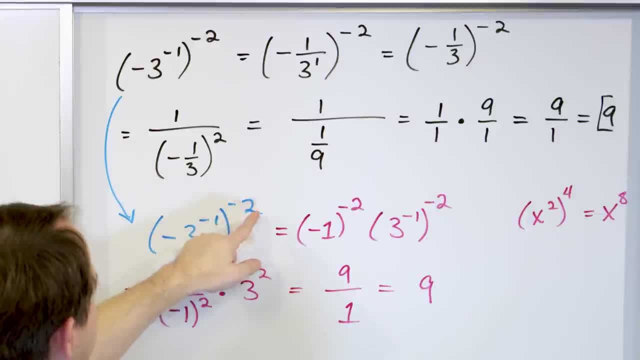 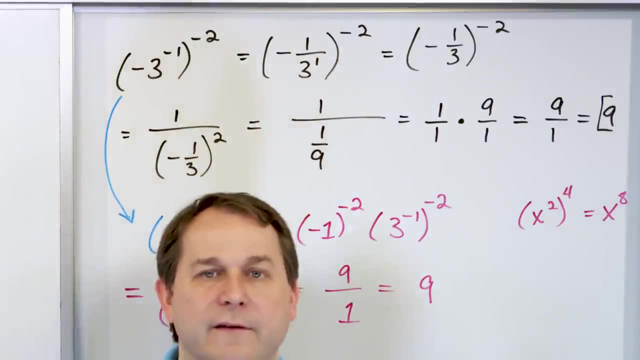 of ways you can do things. If you see it's an exponent raised to an exponent, you can multiply those exponents, Even if they're negative exponents. the answer that you get is going to be the answer you get, Or you can start writing them as fractions and squaring them and manipulating. 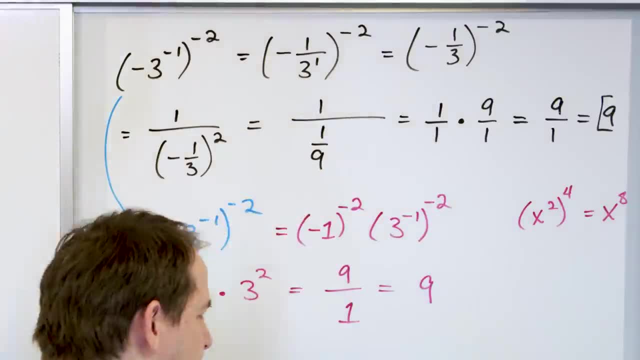 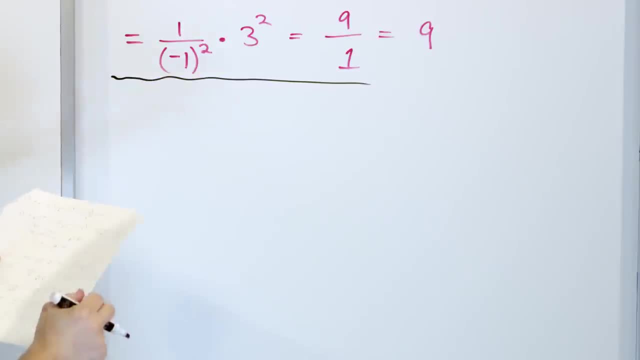 them and multiplying them, and all of that using the same rules of exponents that we've used in the past. If you do things correctly, you will always get the correct answer. Now, what if I have 2 to the negative, 2 power times 3 to the negative, 1 power times 5 to the 0 power raised to the 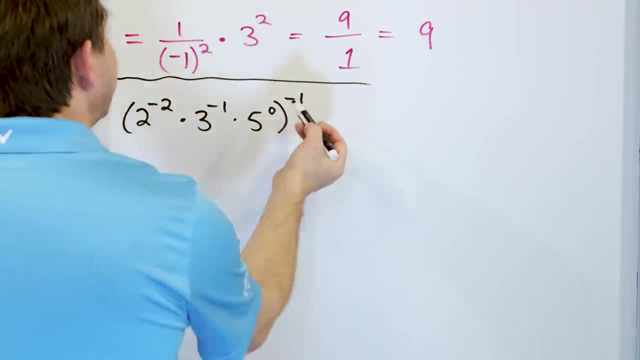 negative 1 power. There's lots of ways to do it. I could take this negative exponent and apply it and multiply it times this exponent and apply it and multiply it times this exponent and apply it and multiply it times this exponent. That's fine, But in this case I'm going to 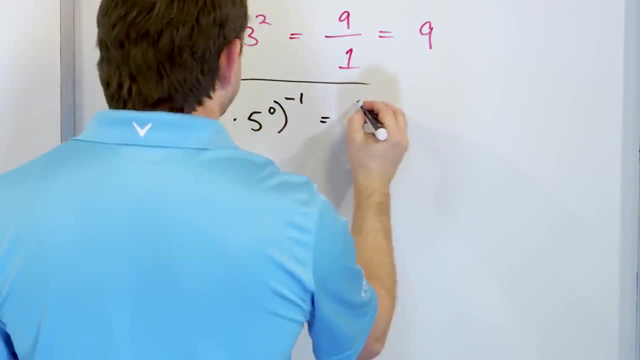 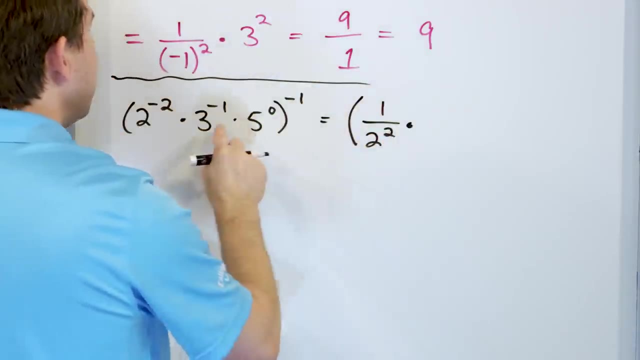 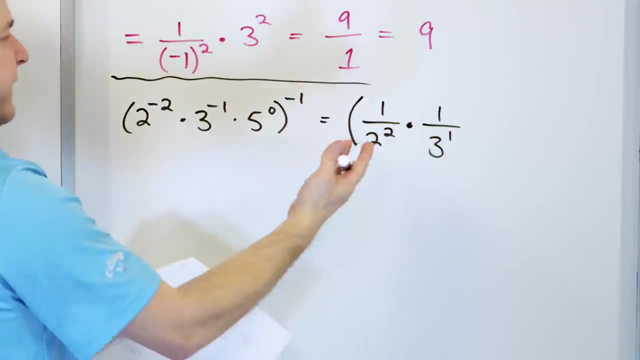 just going to work in the middle. first, This becomes 1 over 2 squared, moving it to the downstairs, making it a positive exponent times. this goes downstairs, making this 1 over 3 to the first power, But 5 to the 0, you always know anything to the 0 is 1.. So 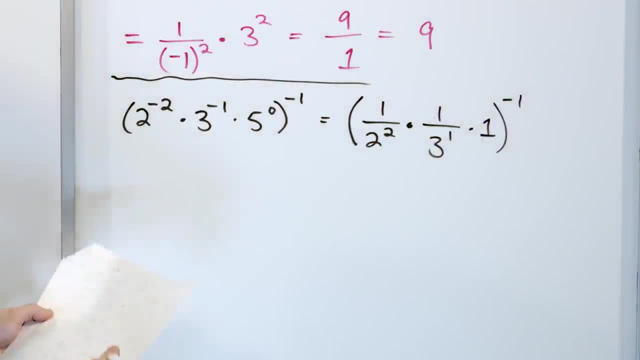 this is just 1.. Now this entire thing is raised to the negative 1 power. So what are you going to have here? You're going to have 1 fourth times, 1 third. You have times 1 there, so I don't need to write that, But it's negative 1.. So let's multiply this. 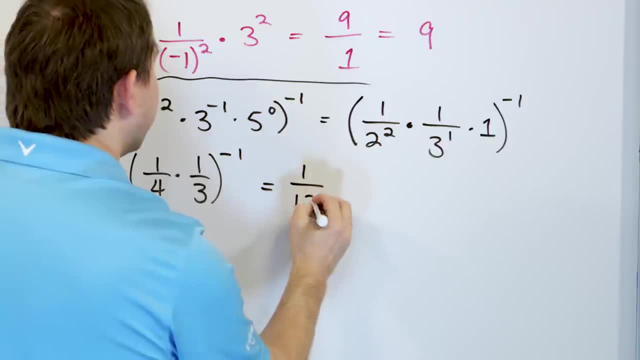 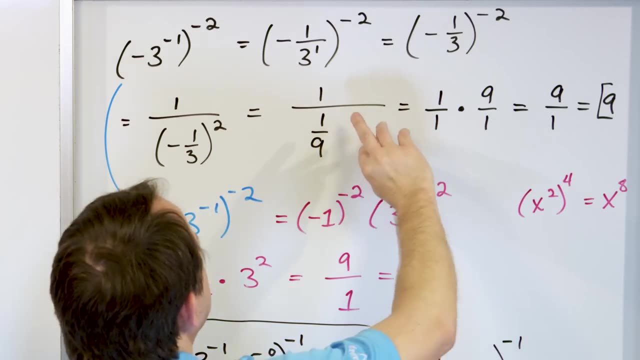 fraction 1. fourth times 1. third: multiply the tops. multiply the bottoms Again, it's to the negative 1 power. So I kind of hinted here that when you have to the negative 1 power, that's what you have here: 1 ninth to the negative 1 power. basically You can: 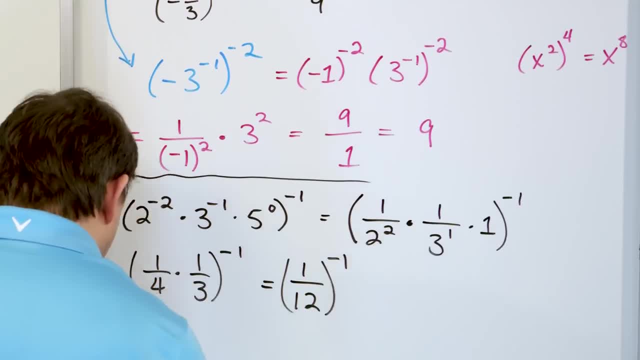 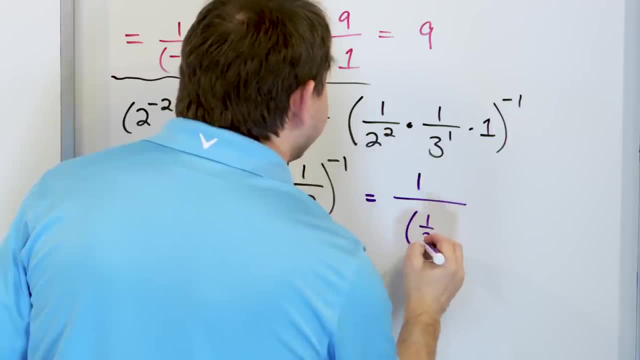 just basically flip it and that's going to be the answer, But I think it's a little bit more clear to show it here. What you're going to have here is, since it's negative 1 power, 1 twelfth to the positive 1 power, taking that negative exponent and moving it down. 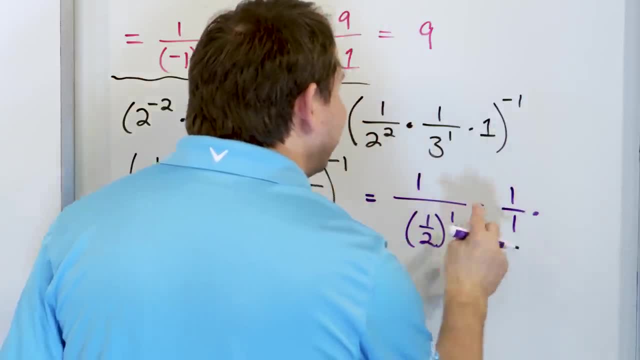 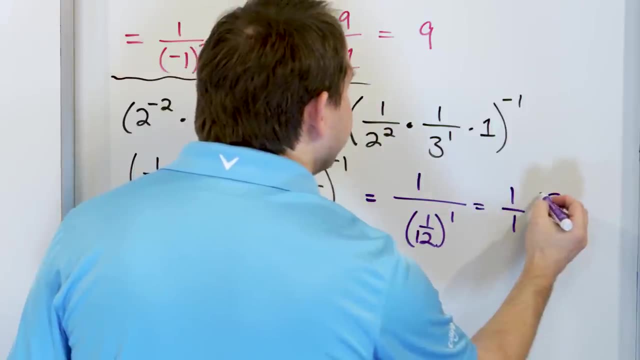 But that means that the numerator is just a number 1 over 1, times. I'll change the fraction division to multiplication. I've got to flip that bottom fraction over to do that. Whoops, this should be 1, twelfth, sorry, like this. And so what you'll get on the top. 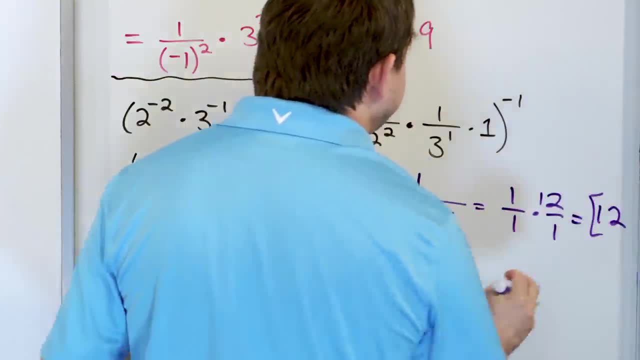 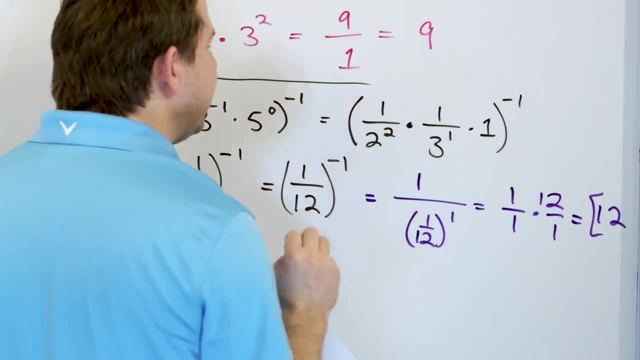 is 12, and on the bottom you get 1,, which means you'll get 12.. And so that's the answer. So again, go ahead and move it to the bottom. Then that fraction division becomes multiplication. Then you get the answer all in steps here, But also in the back of your mind when 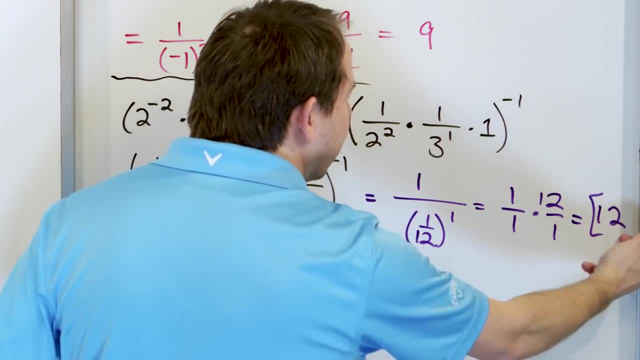 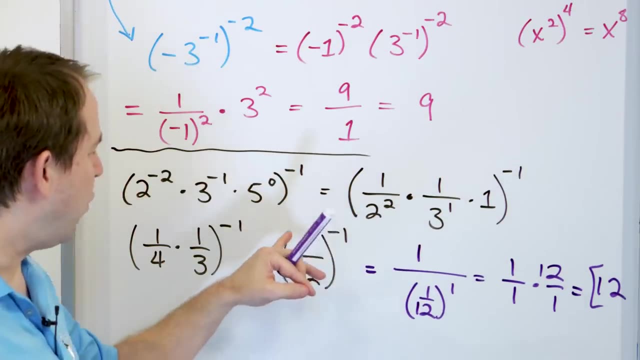 you have numbers raised to a negative 1 power, it ends up just flipping the thing over, giving you 12.. I don't like teaching people to take shortcuts like that, because you can get into trouble. What if it's 1 twelfth to the negative third power? Then you might forget to do something. 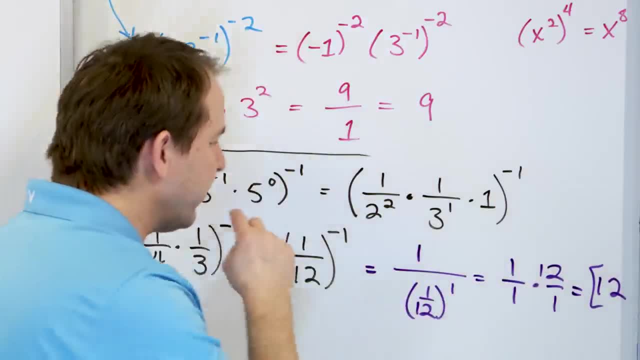 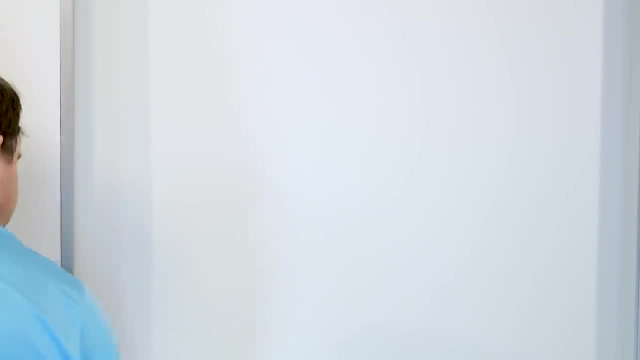 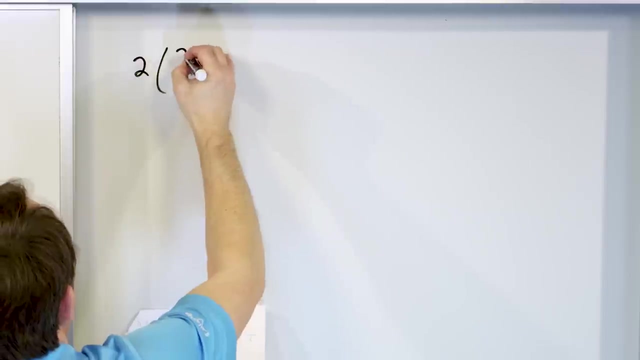 It's better to just move it down, keep the exponent and do everything appropriately, But I am trying to teach you different ways of thinking about these problems. All right, we only have two more One a little bit easier than the other. This one's not too bad. What if you have 2 multiplied? 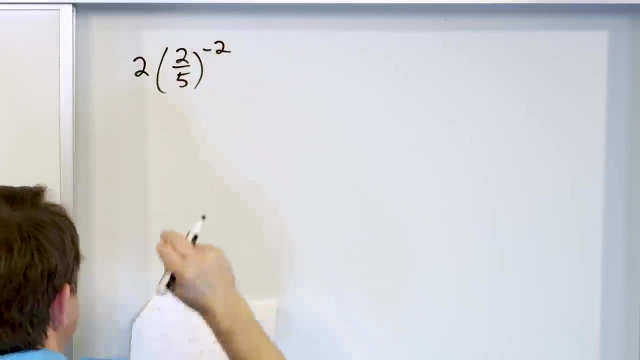 by 2 fifths, raised to the negative 2 power. So again, many, many ways of doing it, but I'm going to do it like this: What if we kept the front here? This is raised to the negative 2 power. so I'm going to multiply that by 1 over the fraction 2 fifths. But that fraction 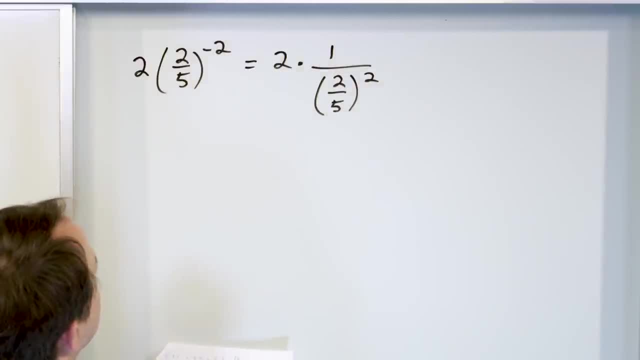 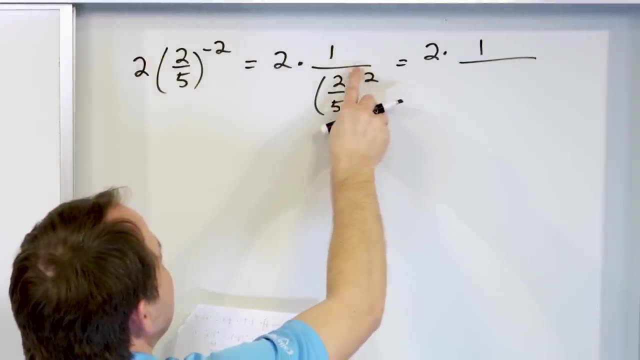 is raised to the positive 2 power. I moved it downstairs, made it a positive guy. here Again it's going to be 2 times 1 over. this is a fraction raised to an exponent. The numerator is raised to the power of 2.. The denominator is also raised to the power. 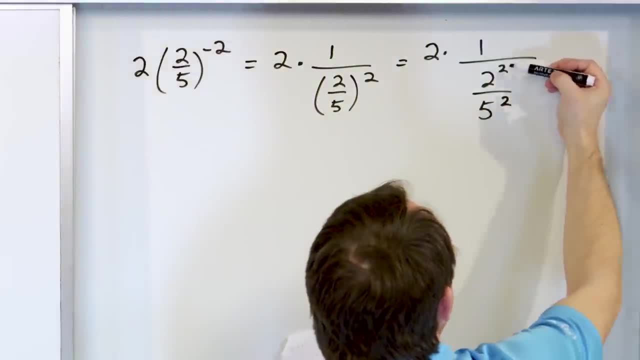 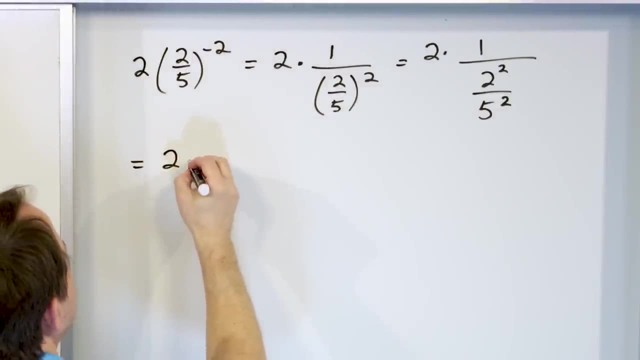 of 2.. I know that you don't like the idea of having an ugly fraction like this in the denominator of a larger fraction, but you're going to have to get used to it because it's just like that in algebra. So let's keep the 2 times here In the bottom: 2 squared is 4, 5 squared. 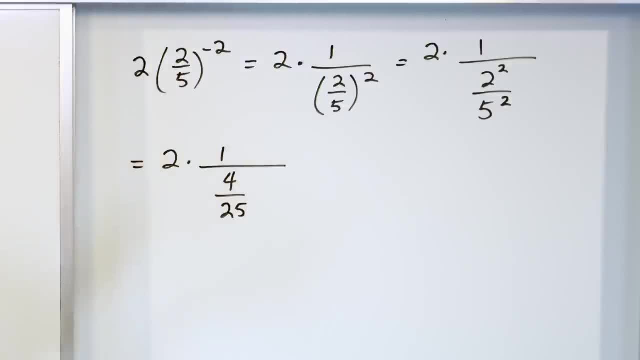 is 25.. So there's a couple of ways to proceed, but basically let's keep the 2 out in front here. Now, this is fraction division. It's a number divided by a fraction, So let's write this as 1 over 1 multiplied by, because that's what it is. 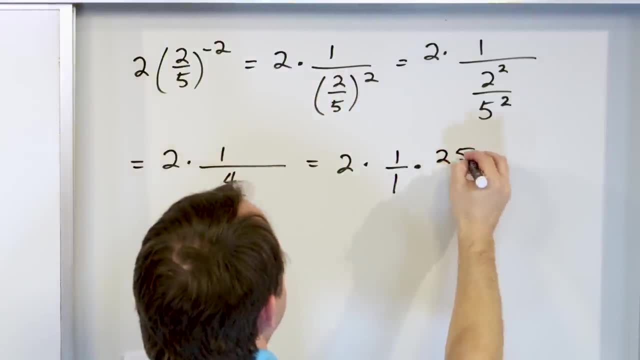 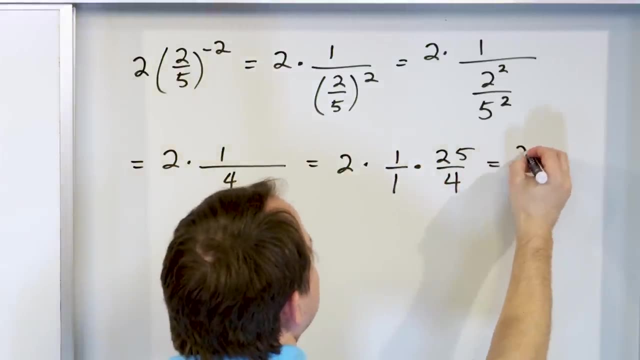 1 over 1.. We'll take this, we'll flip it over and multiply 25 over 4.. So you see what's happened. You have 2 times this times this. So what you really have is 2 over 1. from this times 1 times. 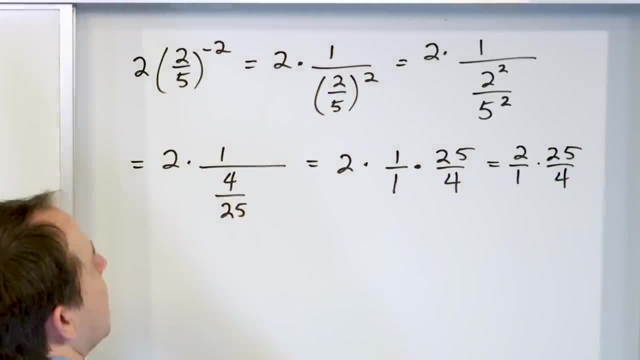 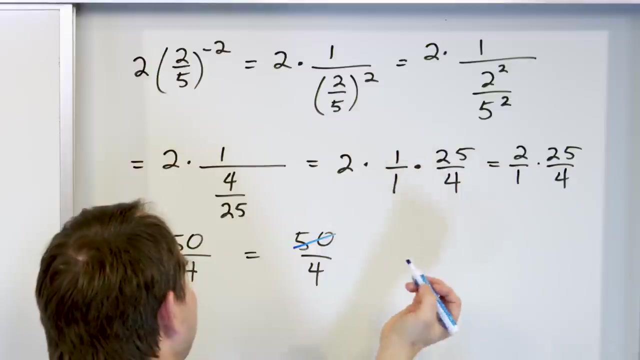 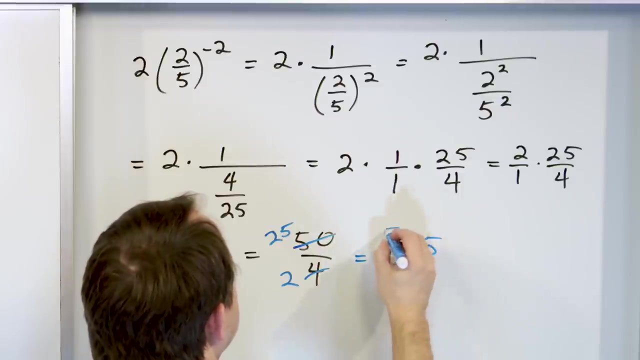 25 over 4.. Now you multiply the numerators together, giving you 50.. Multiply the denominators together, giving you 4.. And then 50 over 4.. You need to think of something to divide top and bottom by 50 divided by 2 is 25.. 4 divided by 2 is 2.. So 25 over 2.. Final answer: I can't divide. 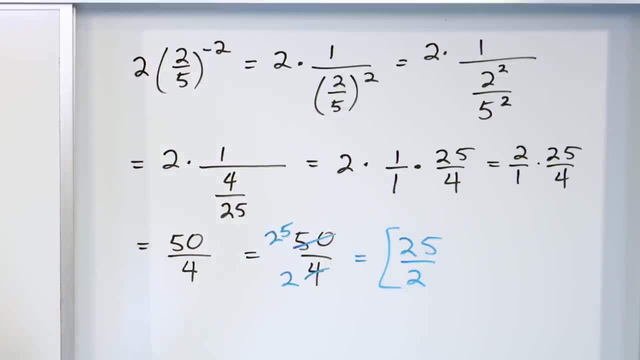 top and bottom by anything common anymore. 25 over 2 is the final answer. There are several places through this that I could actually think right now off the top of my head to do it slightly differently, getting the same answer. This is the way I did it when I did it the first time. 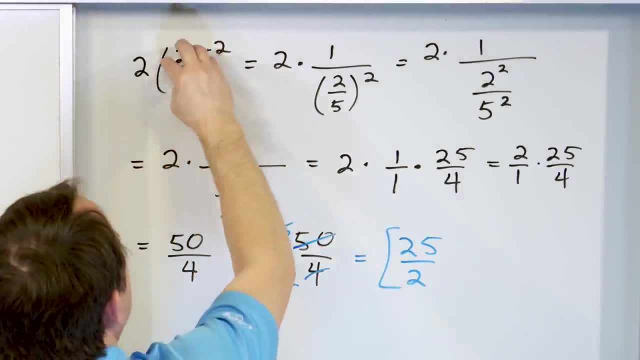 But just looking at it again, another way to go is, instead of rewriting this down below, you could take this fraction and you could distribute the negative 2 as an exponent to the top and then the negative 2 as an exponent to the bottom, And then continue to simplify it that way. 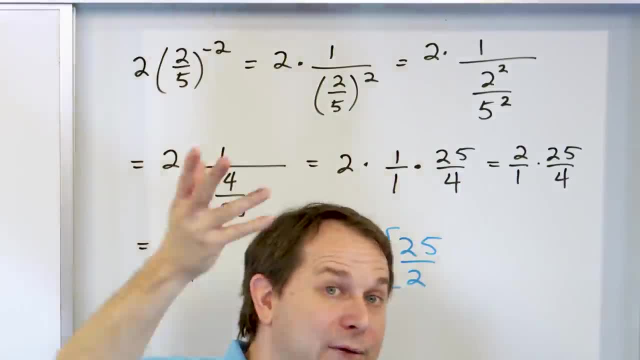 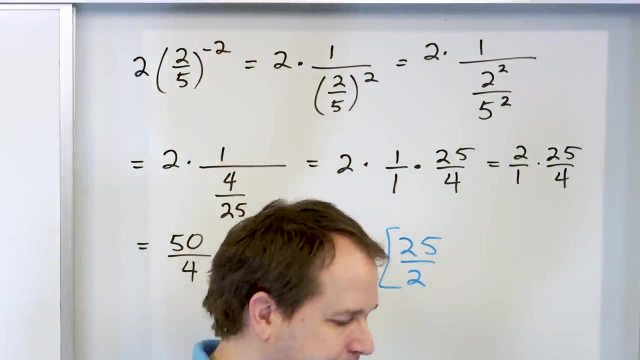 But then you would have two negative exponents and it would be more fractions divided by more fractions And you would get there. You would definitely get the right place, But it would be a slightly different answer. It would be a slightly different path than the way we took it Now. so far, all of these problems. 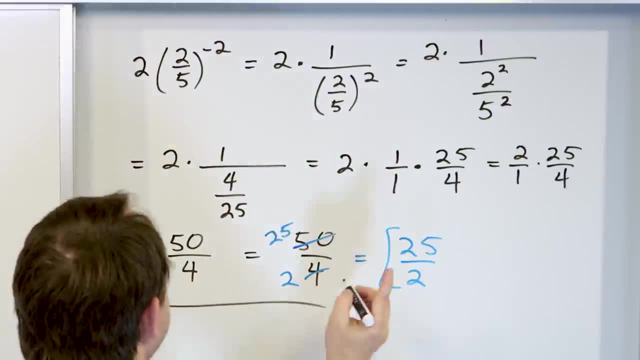 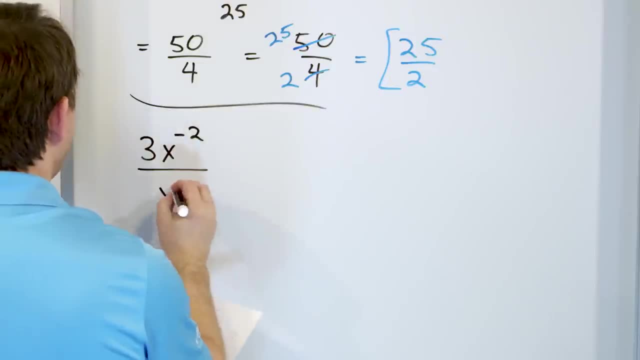 have had just numbers, I would like to, in this section, at least do one problem involving variables with negative exponents. So here we go: 3 times x to the negative, 2 divided by y to the negative, 1.. Now, before learning about negative exponents, this looks terrifying to most people. 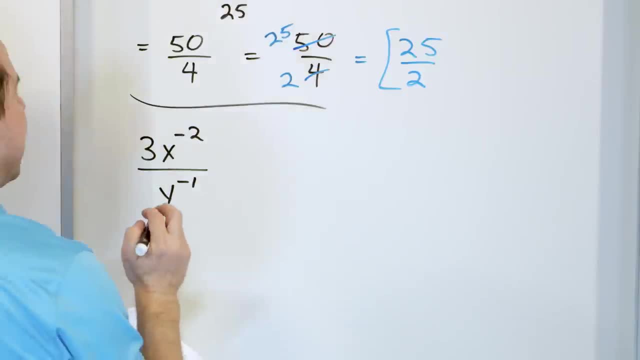 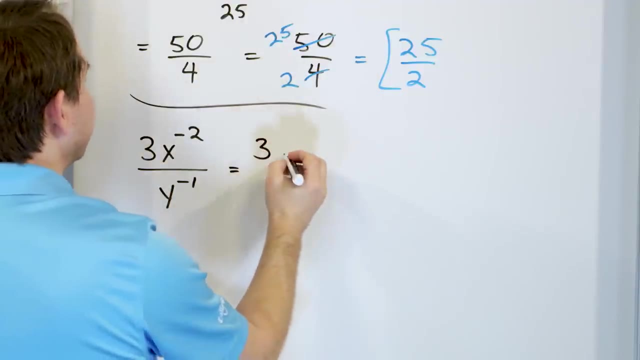 It just looks ugly with the negative exponents here. But now I want you to take it one step at a time. We know that x is raised to the negative 2, so we write that as a fraction. I know it's ugly in the beginning. You don't want to do this stuff, But what you end up getting is three times. 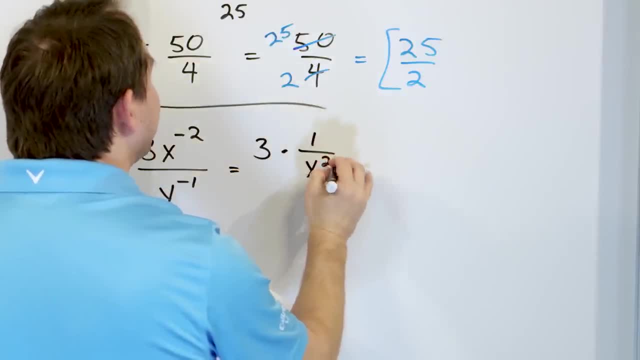 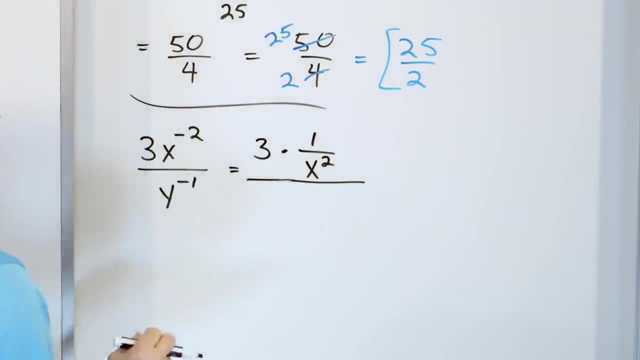 you move this into a fraction 1 over x squared, making it positive. But this whole thing lives in the numerator of a larger fraction. So I draw a larger fraction line down here And then the bottom. I make this a fraction 1 over y to the first. I've turned this into a fraction. I've 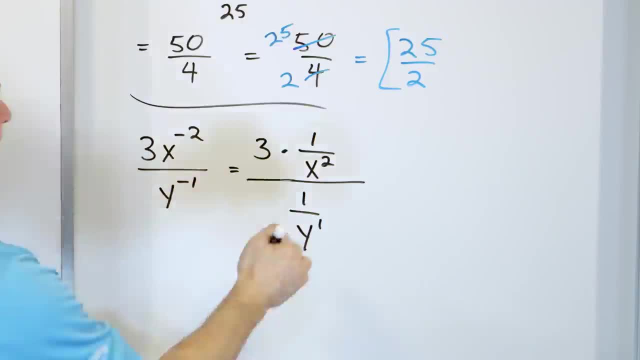 turned this into a fraction. I've preserved the structure of the original thing. Yes, it looks ugly. You're just going to have to get used to that. Now, on the top it's going to basically be 3 over 1 times this. So you multiply the tops 3. Multiply the bottoms: x squared, Because you're. 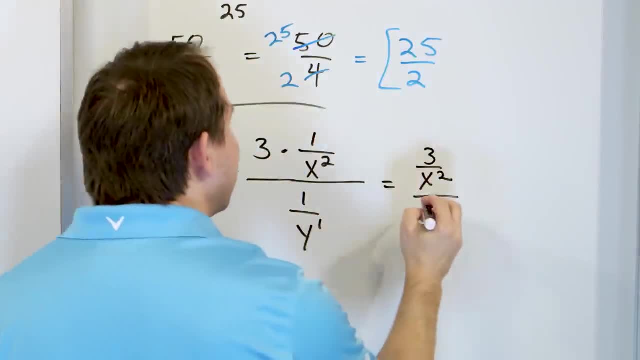 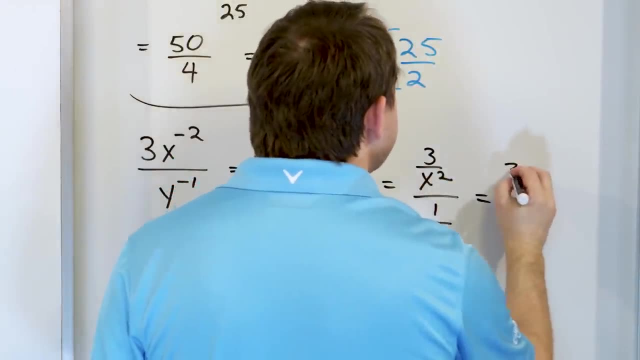 taking 3 over 1 times this. multiply tops, multiply bottoms. On the bottom you're still going to be stuck with the 1 over y. But then you have a fraction divided by a fraction. We know how to handle that. You take the top fraction, change this division here to multiplication. take the 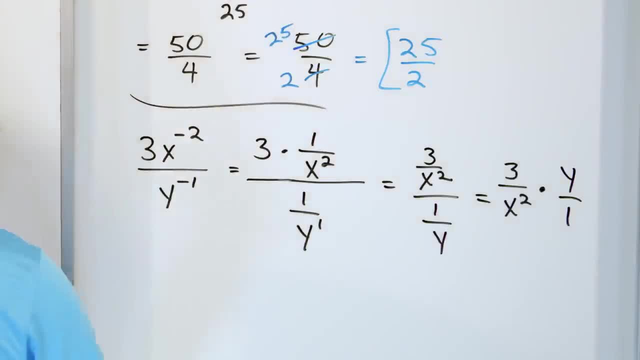 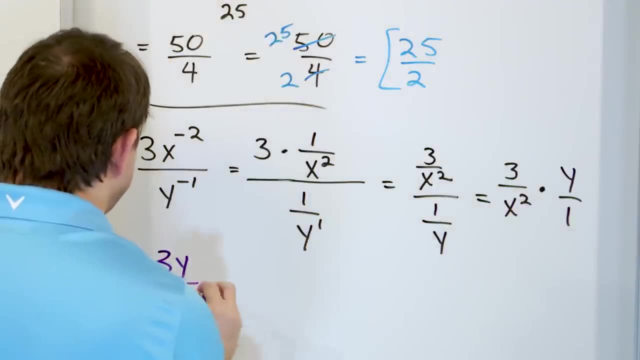 bottom fraction. flip it over And then we can now finally multiply them 3 times y. we'll give you 3y, And then x squared times 1, we'll give you x squared, So you get 3y over x. 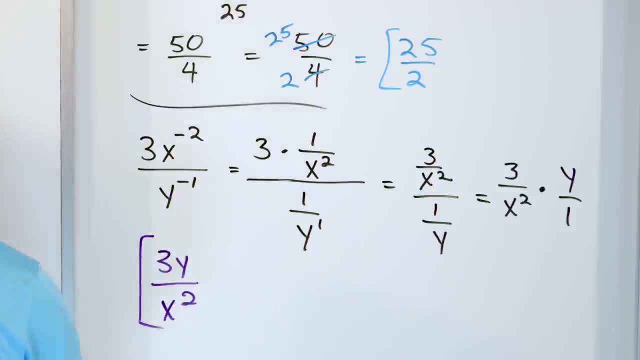 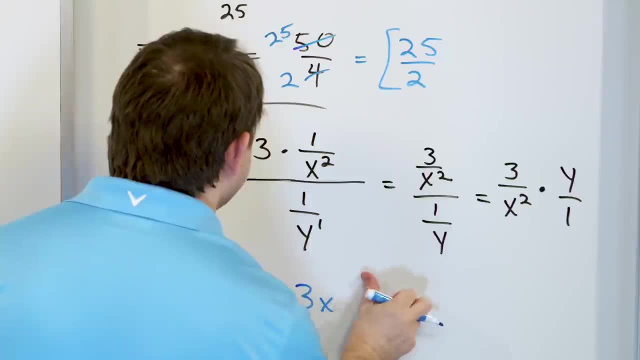 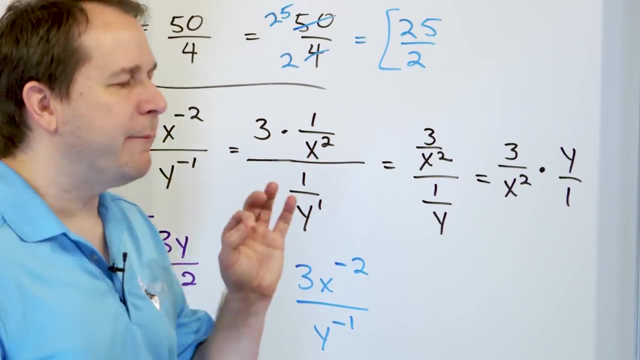 squared. This is the final answer. Now, one more thing I want to say about this problem before I move on is the following: Let me rewrite this problem statement again: 3x squared- whoops, not x squared. 3x to the negative 2, y to the negative 1.. Now, so far I've been describing 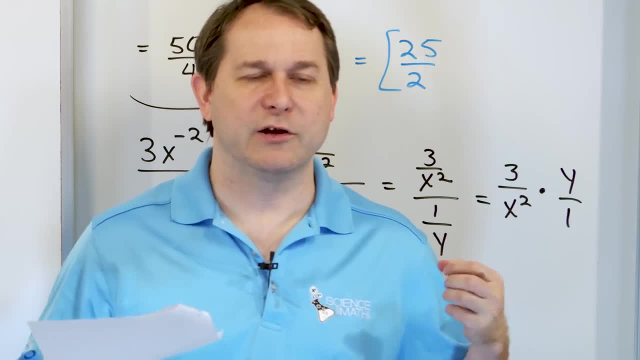 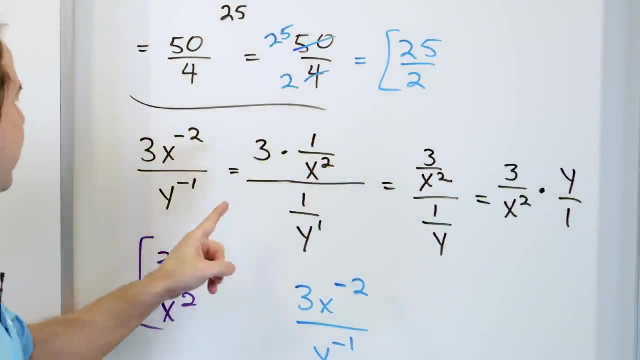 all of this stuff as a very cookie cutter, kind of like learning how to cook in the kitchen. You don't want to do this before the other, right? Because I want you to get those skills. I said: turn this into a proper fraction with a positive exponent. Turn this into a fraction like this: 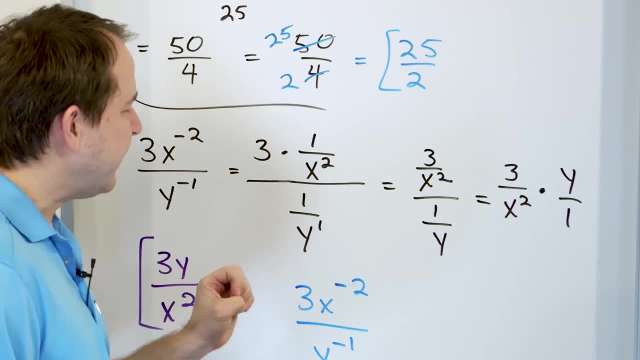 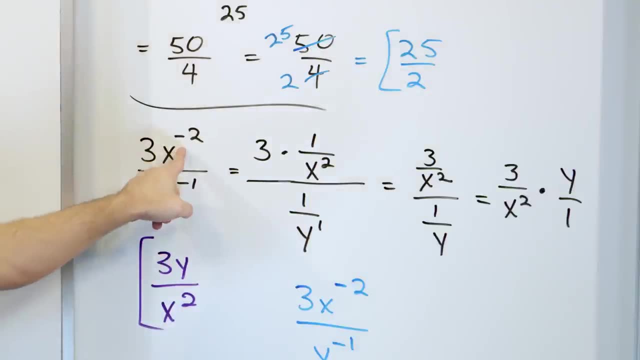 Go through the whole thing. Simplify it, OK, fine, But now I want to take the training wheels off just a little bit here at the end of the lesson, to kind of open your mind a little bit. Just like we said that we take these guys and we write them as fractions. It's not really a shortcut. 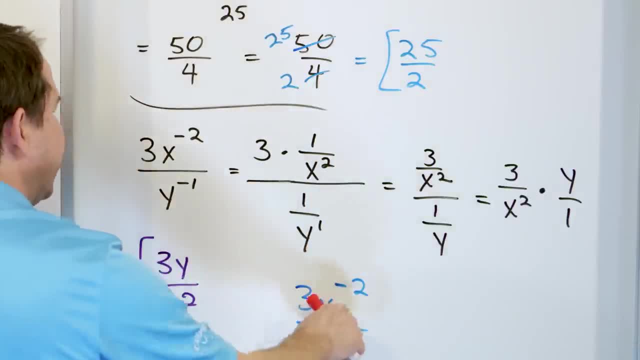 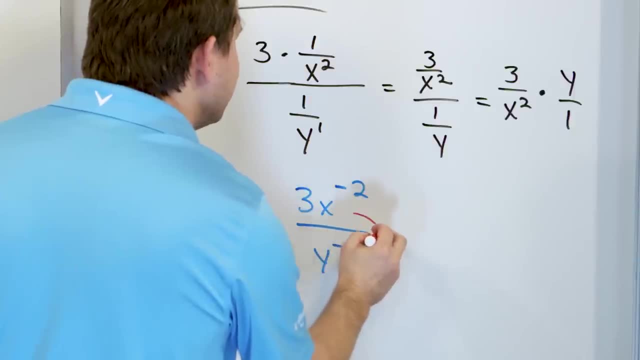 but it's another way of thinking about it. What happens here? in the top? you have a negative 2 power. So what you could do, but without doing any of these steps, is you could take this x to the negative 2 term and you can move them downstairs. 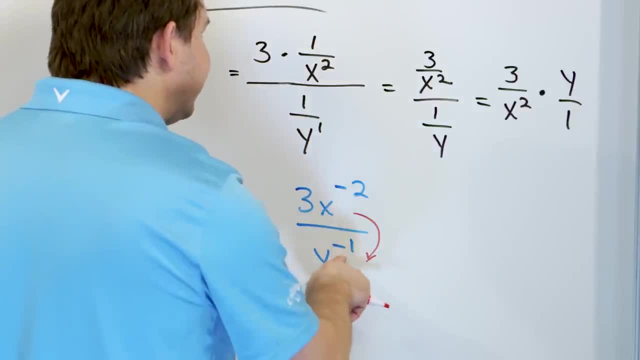 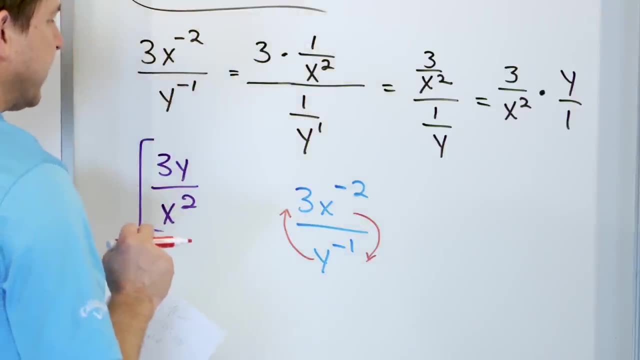 making it a positive x squared, But then you have this negative here as well. When you have a negative in the bottom, it ends up working out that you can move him upstairs, making him positive. So if you follow that kind of rule, then what's going to happen is you're going to take this and 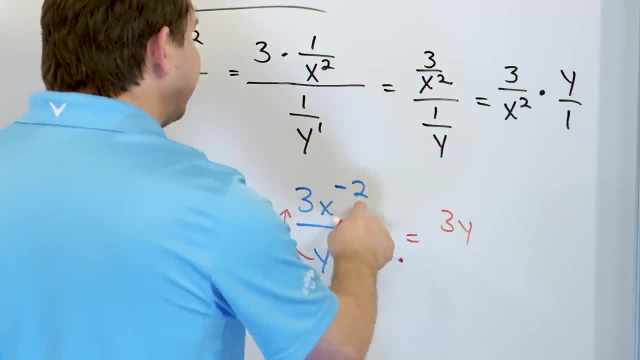 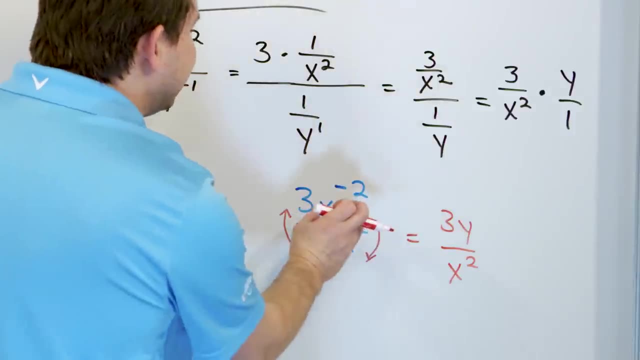 move him upstairs, making it 3 to the positive y, And you'll take this and move him downstairs, making him x to the positive 2, which is exactly what we got in the answer. We can easily see why you can move this downstairs, because that's the definition of what we've been doing. We've 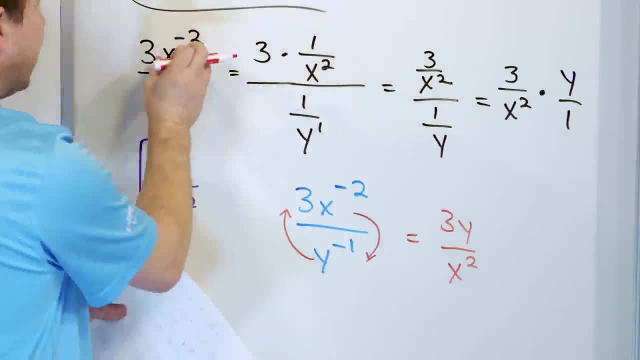 been taking these like this and we move them downstairs. But it also works with the bigger fraction. You just move the whole thing downstairs, making it a positive exponent. But it also works out that you can take these upstairs and make them a positive exponent. 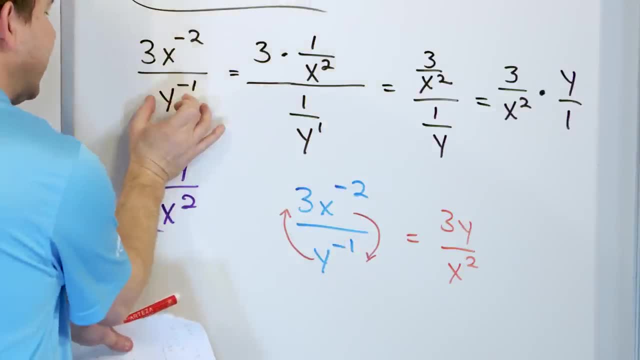 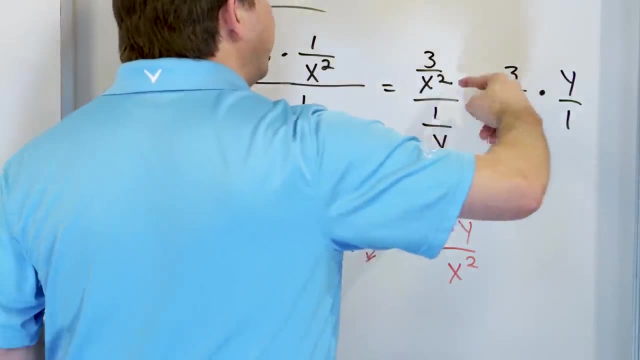 Why does it work that way? The reason it works is because if you have a negative exponent in the bottom, it's exactly the same thing as a fraction in the bottom, And anytime you're dividing by a fraction in the bottom, it always works out that you can flip them upstairs, retaining. 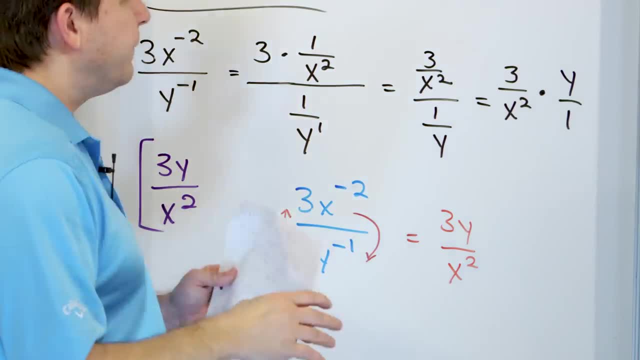 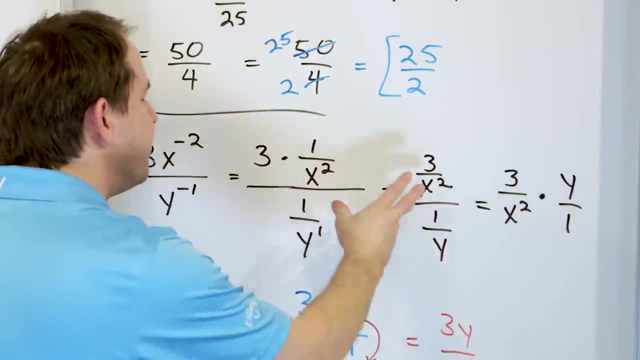 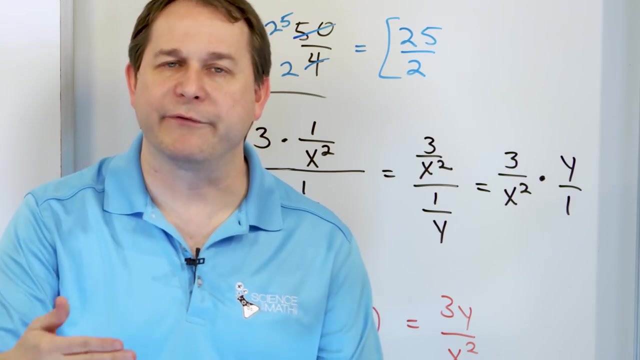 his power in the top. So there's multiple ways to do problems in algebra, The way I'm teaching you here. put this into a fraction. put this into a fraction, multiply, manipulate, get the right answer. But it's equally a good idea, as we go on through problems, for you to recognize patterns. 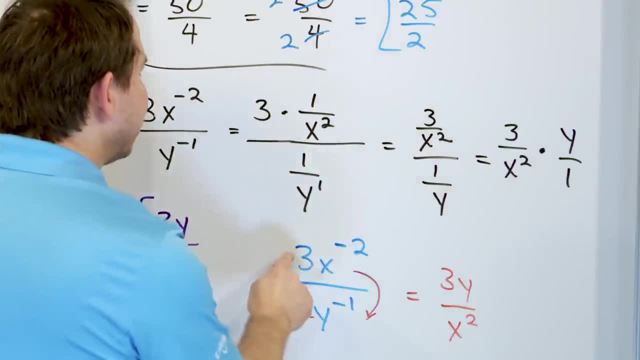 and see that what's going to happen as you get more experience with this is you're going to have all of this here and all of this here. This negative exponent will just simply be moved downstairs and made a positive exponent, And this negative 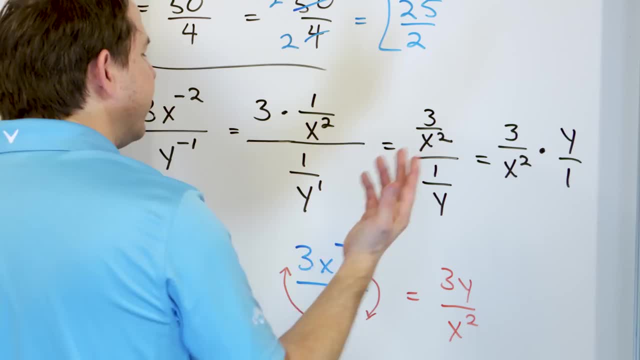 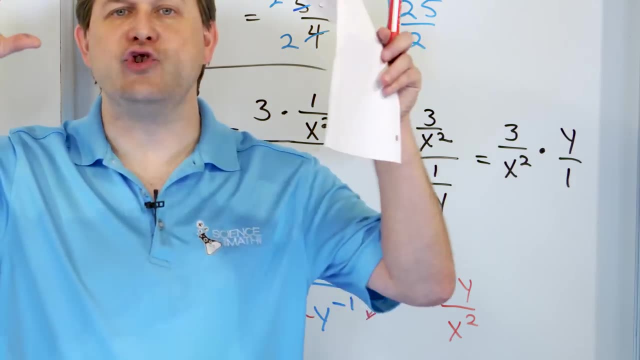 exponent will have to be moved upstairs And that works because of the fraction division. So bottom, bottom, bottom, bottom, bottom bottom line is: if you see negative exponents in the numerator of fractions, you can grab them, move them down below, making them positive. 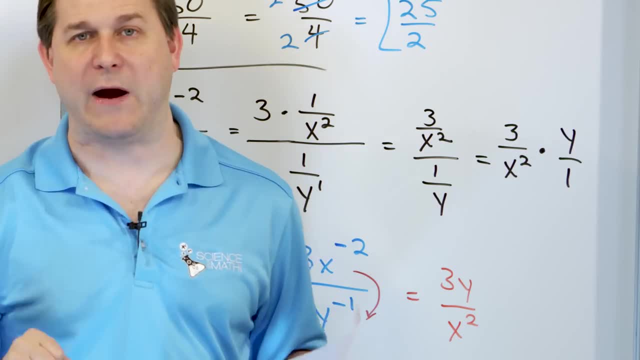 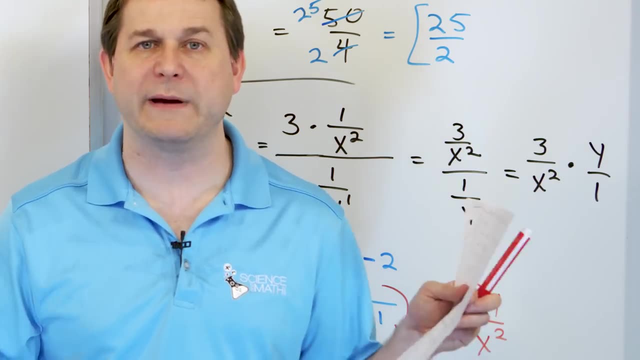 exponents. If you see negative exponents in the bottom of fractions, you can grab them, move them upstairs making them positive. That doesn't work because it's a shortcut. It doesn't work because it's black magic. It works because of what we've done in this problem. 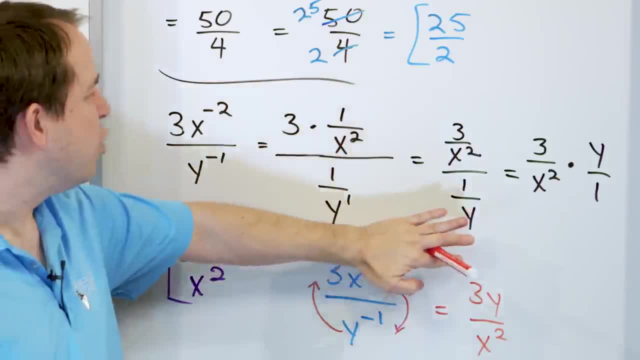 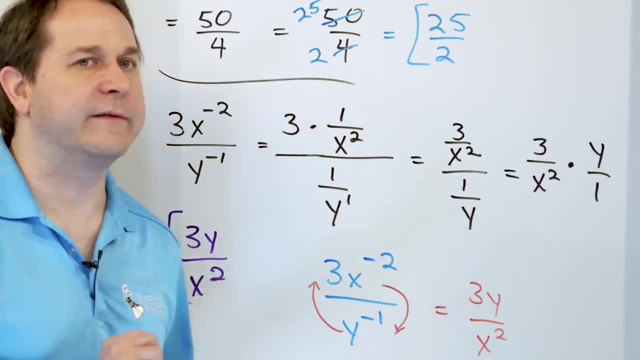 These negative exponents become positive and these in the bottom become positive. When you do the multiplication, the ones in the bottom get flipped over anyway. So that's why you can move things around like this. Sometimes you'll see some books teaching it like that. I'll do kind of a mixture as we go, I'll show you the long way and I'll kind of 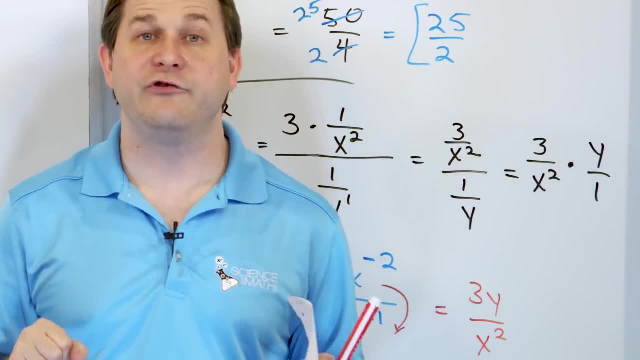 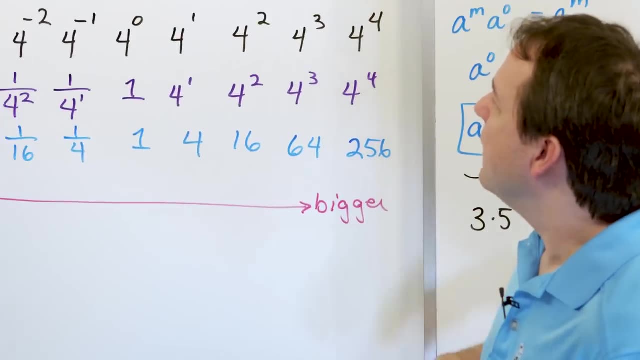 remind you: hey, you can move that there, You can move this here, making the exponents, changing them into positive exponents. So, really, if you wanted to revise things- and some books actually do this- you could say: if I have a negative exponent at the top of a fraction, 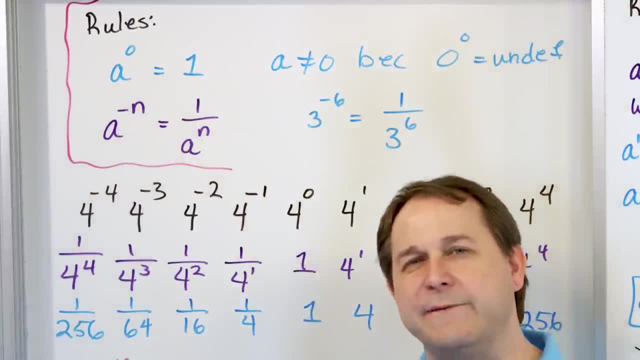 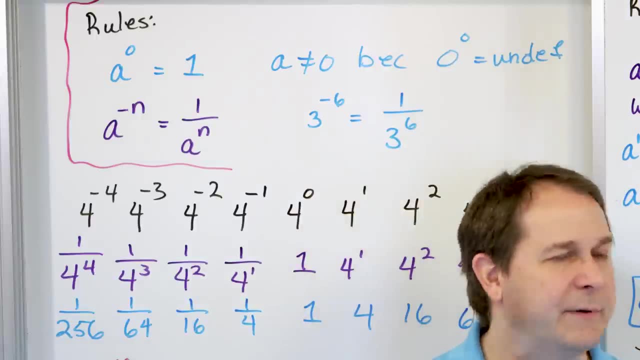 move it to the bottom with a positive exponent. If I see a negative exponent in the bottom of a fraction, move it to the top with a positive exponent. That's fine. You can think of it that way if you like. I'm going to end up solving the problems a couple of different ways to give you. 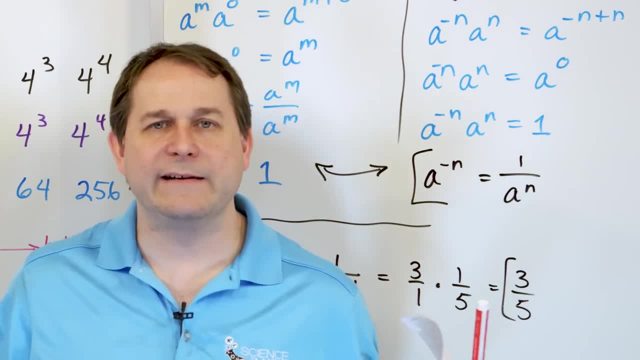 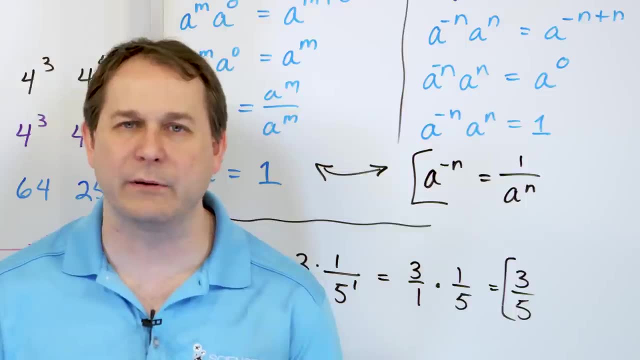 flavor of how to do this stuff. If you've had any difficulty with this lesson, watch it again. please Go through it yourself. Make sure you understand it. You have to learn so many things here. You have to learn about negative exponents. You have to learn about zero exponents. You have